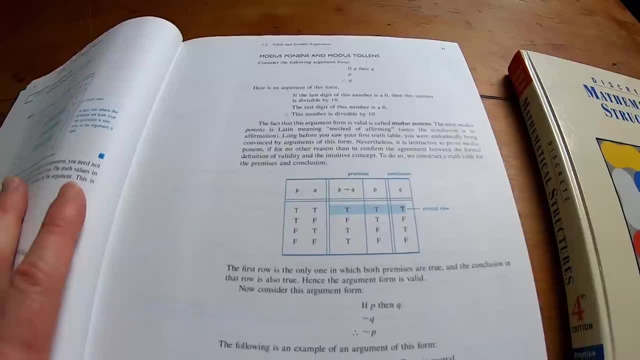 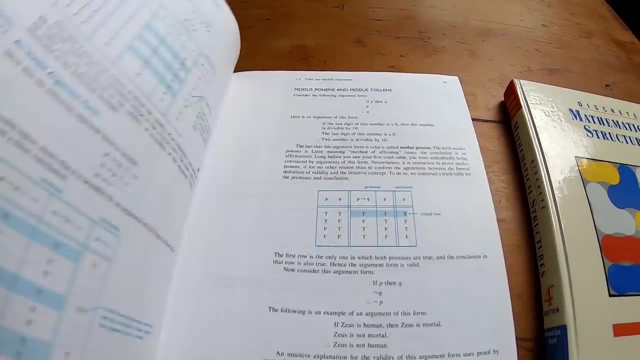 And the beautiful thing is, you need zero algebra to learn this Now. you will have to learn algebra at some point and I'll show you later in the video, but you can start with this. You can start off by taking a look at the core foundations of mathematics. It's really, really. 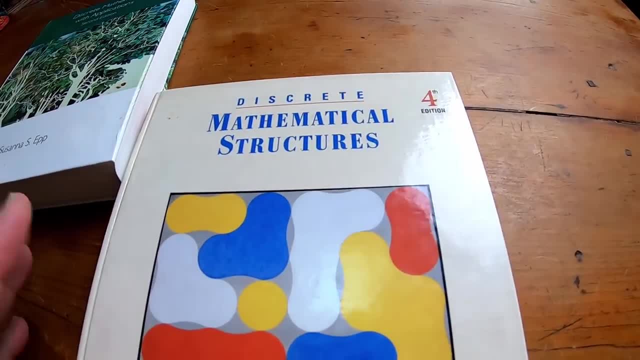 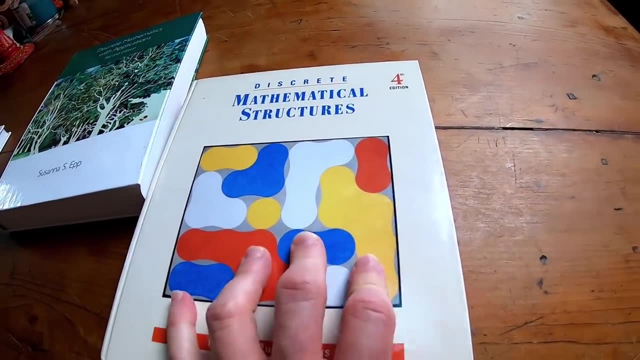 quite beautiful. This other book is just another book on discrete math that I have- and I have, like you know, 10 of these- But these two are really good for beginners and that's what this video is about. right, You want to get started and you want to learn. This is the book by Coleman Busby. 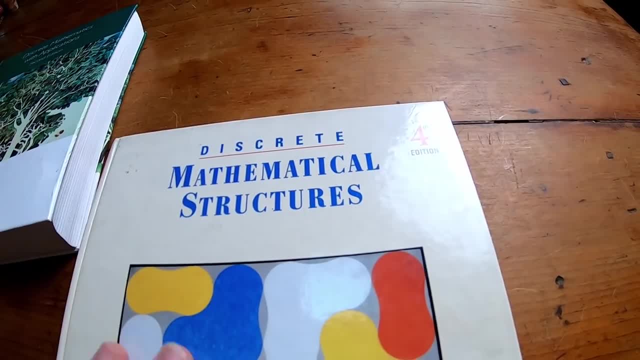 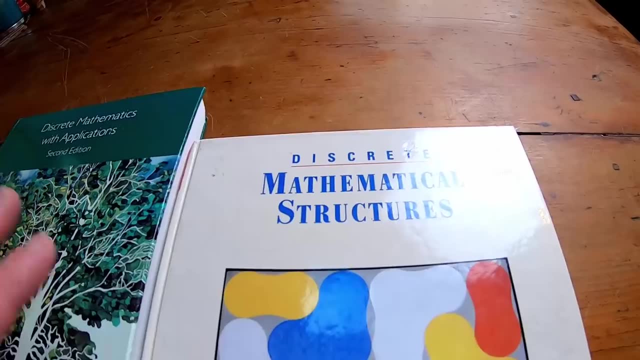 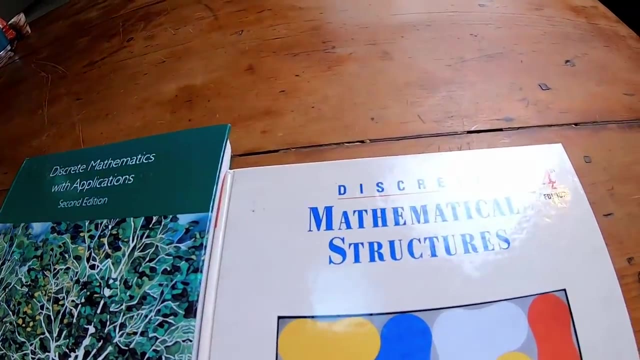 and Ross, and this is also a very, very beginner friendly book on discrete math. So in discrete math you learn all kinds of stuff like logic sets and you learn how to write proofs. You also to learn other more advanced topics that you typically don't see in other classes, like calculus. 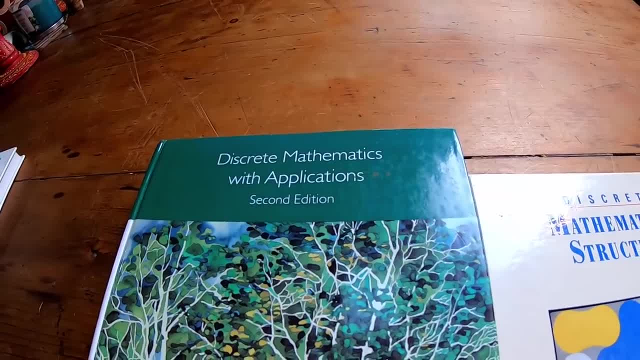 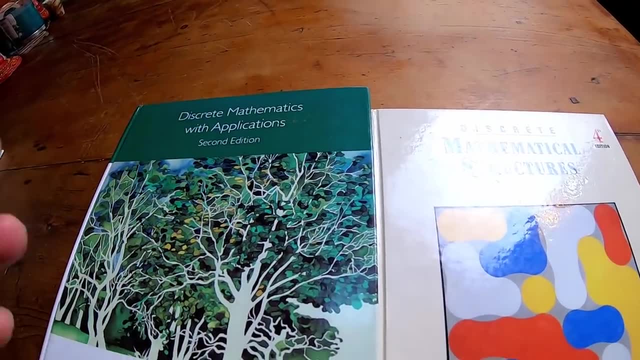 and stuff like that. So you learn a lot of really cool math that oftentimes math majors don't even see. So it's a good place to start and a good place to keep you motivated to start at the beginning, Because you've probably done algebra in the past, Maybe you were in school before, Maybe 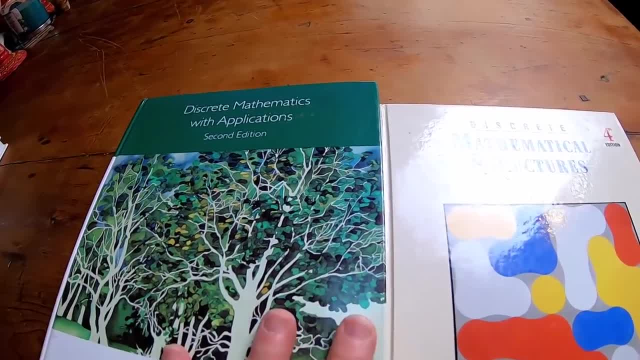 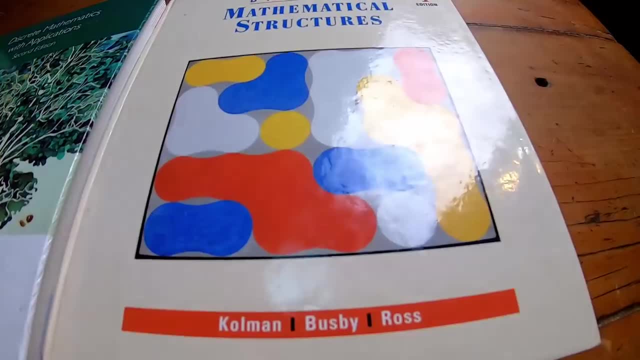 you're in school now And we just do so much algebra, So I think that this is a really good starting point for people Discrete math especially this book- the one by Epp and the one by Coleman Busby and Ross is also pretty good. This one is better, though This is probably a really good. 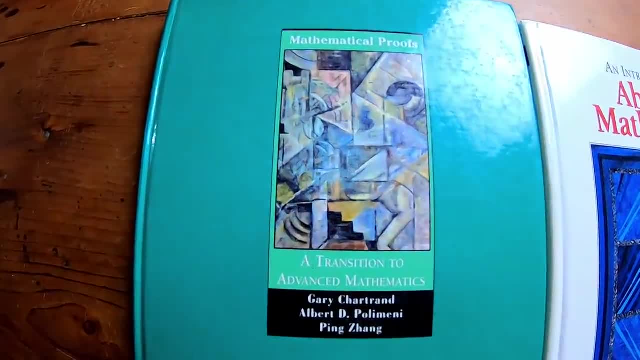 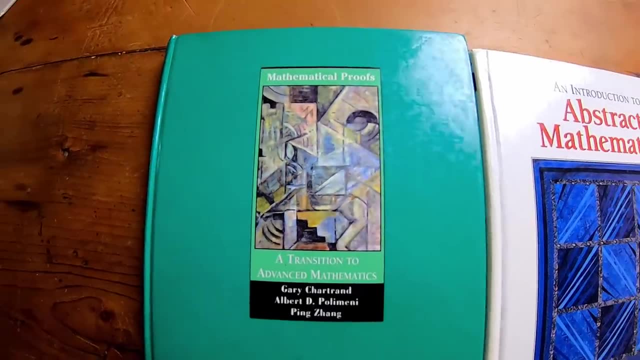 choice. So here we have two proof writing books. This is Mathematical Proofs, A Transition to Advanced Mathematics. This is the Chartrand, Polimini and Zhang book. This book is awesome. Now, this is way more advanced than the previous book. So you know, you pick up these books, you read what. 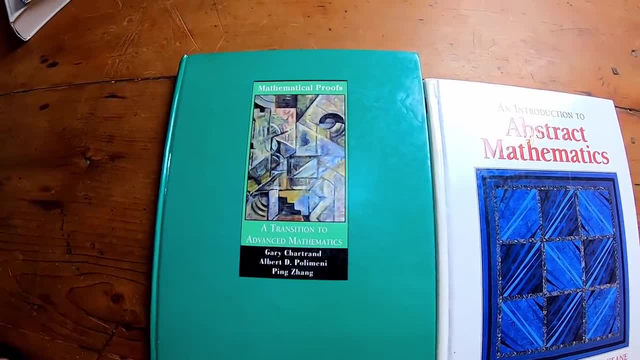 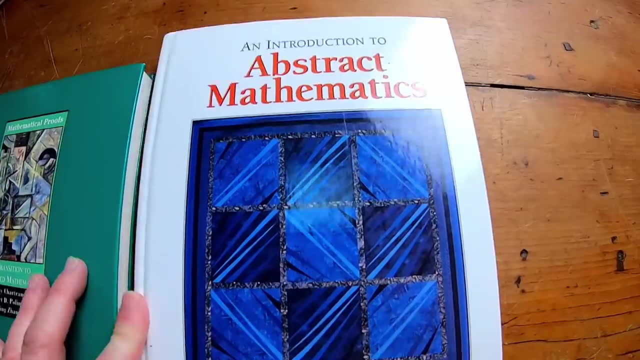 you can and you try to understand them, And you try to understand them, And you try to understand as much as you can, And then you move on to the next topic. You're not expected to master everything in any of these books, by the way, And this is another book on proof writing. This is the. 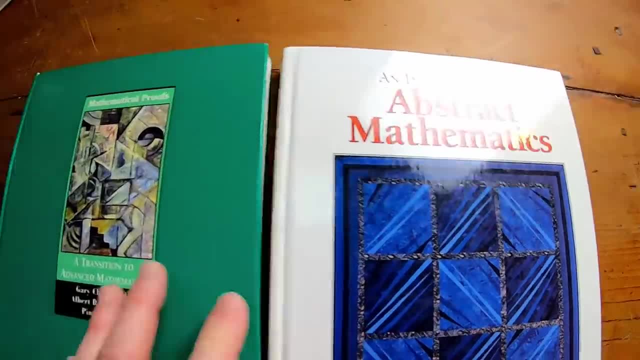 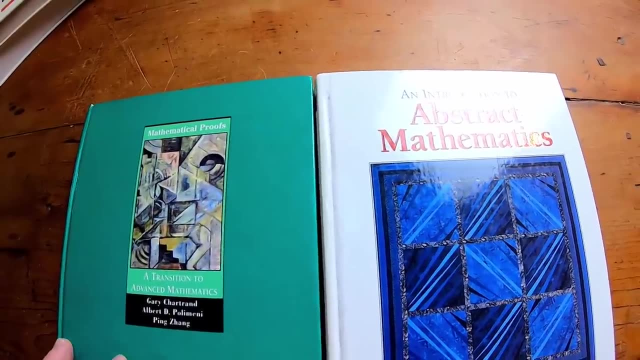 one by Bond and Keene. This one is also good, but this one is better. And, by the way, every book I'm showing so far here you can probably get it for less than $10 on the internet if you get a used. 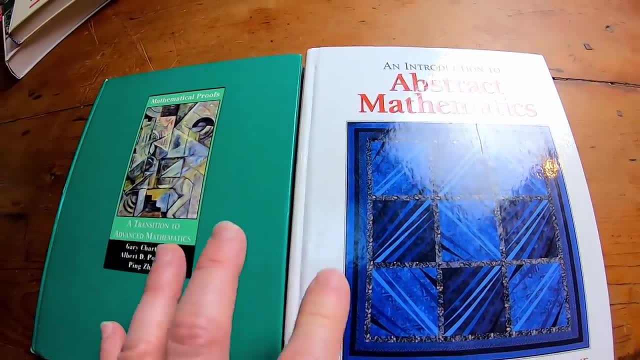 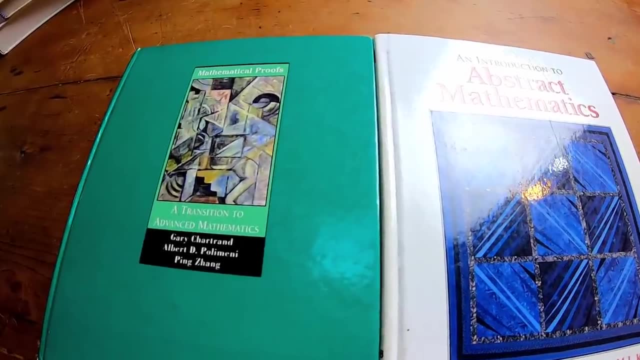 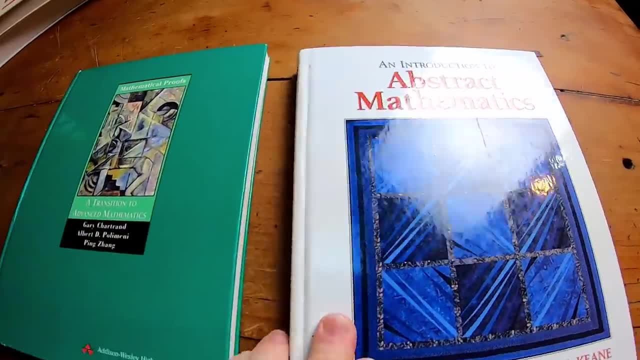 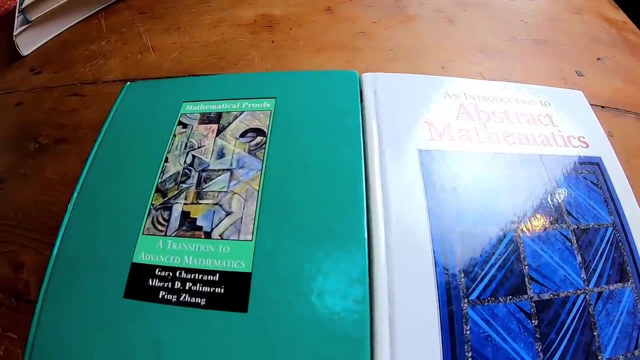 to write proofs, And these two little books basically teach you how to do that. So, again, you're not expected to. you know completely, master everything in these books, So just make an effort. Why are there pre-algebra books in this video? Well, remember, this is from start. 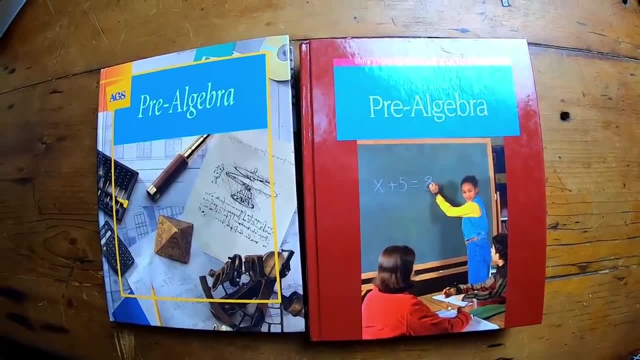 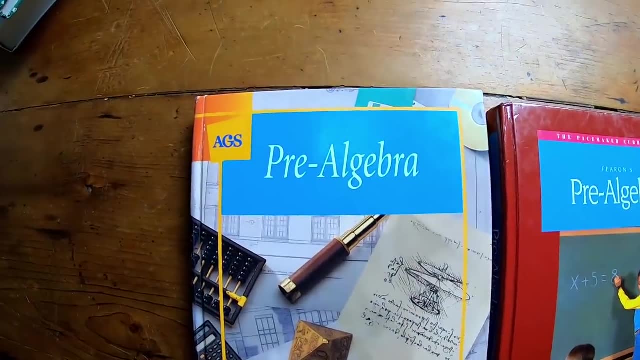 to finish. So, once you've attempted those books and you've learned some logic- and maybe that's all you've learned, maybe your math is really bad, So maybe you need some pre-algebra. So these are just two pre-algebra books that I have that I like. This is the one it says AGS. 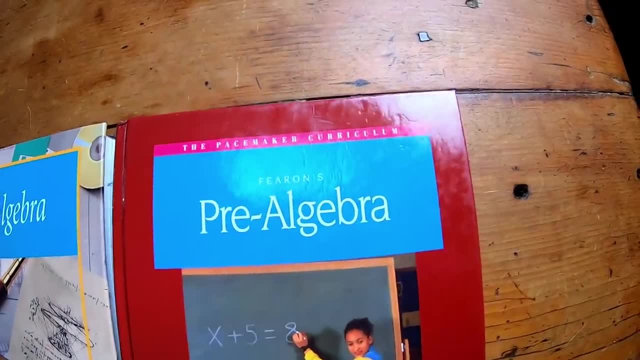 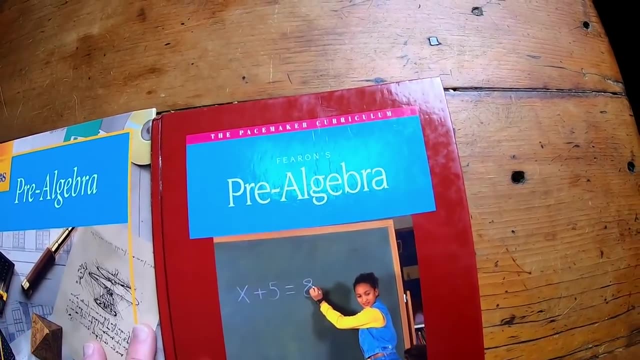 This one's good because it has solutions And this is Fearon's pre-algebra. This one doesn't have solutions, but I actually like this one better than this one. So if you're just trying to like refresh really basic math, these are two pretty good pre-algebra books. I have about 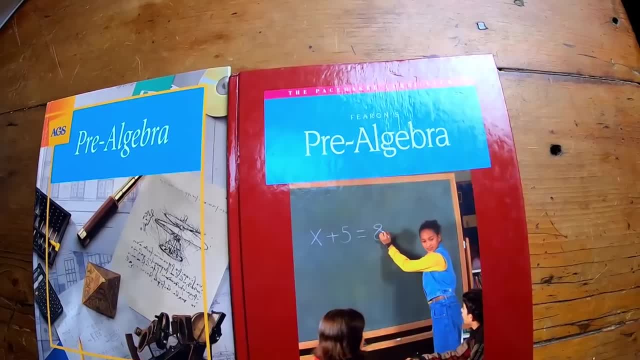 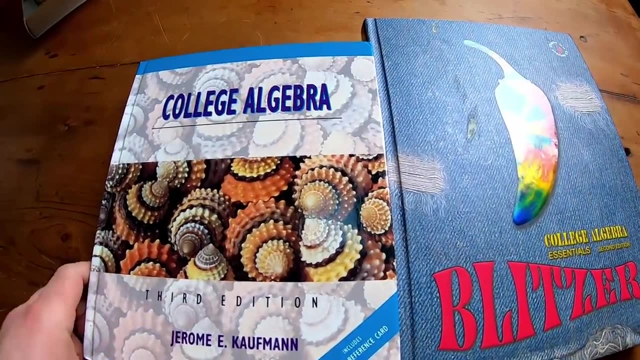 eight pre-algebra books and I think these are maybe the best ones. So maybe you decide you don't need pre-algebra or you've already worked through it and you feel good enough about the material. Then college algebra is a good next choice. So college algebra is a course where you 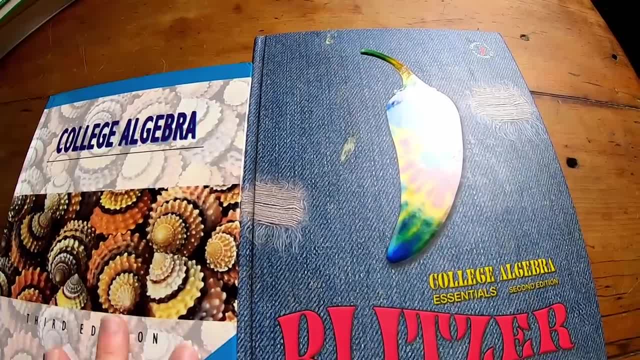 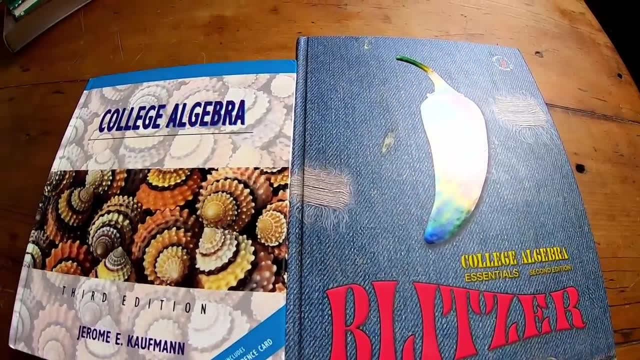 learn just basic algebra. There is a course in between these called intermediate algebra. I decided to skip that one because most intermediate algebra books just contain like just thousands of problems and it's just too much. These books, I think, are better and they're better written. 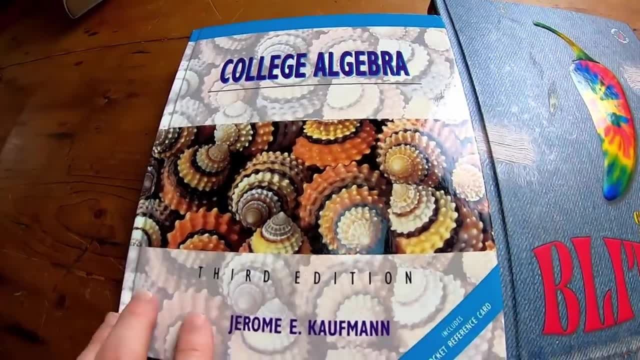 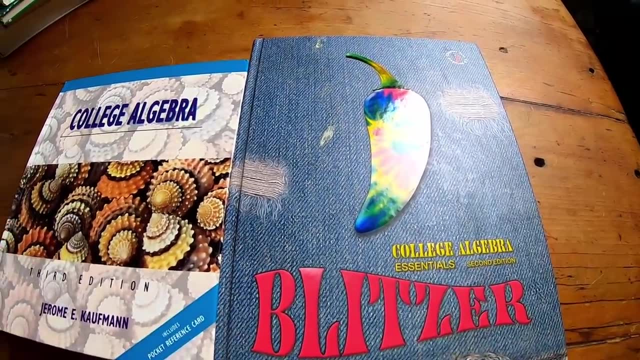 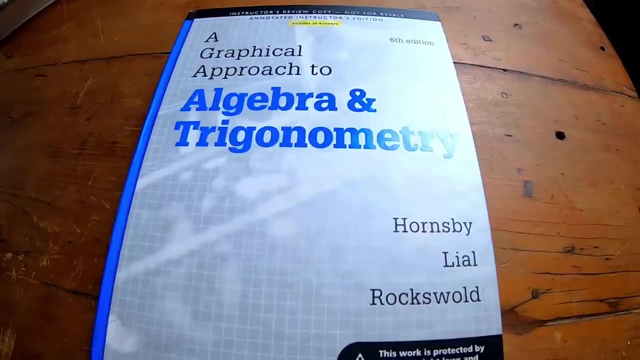 So this is the one by Kaufman. It's a little bit more beginner-friendly than this one. This is the one by Kaufman. It's a little bit more beginner-friendly than this one. So this is the one by Kaufman. Once you get through college- algebra or like- you feel like you've mastered enough of the material. 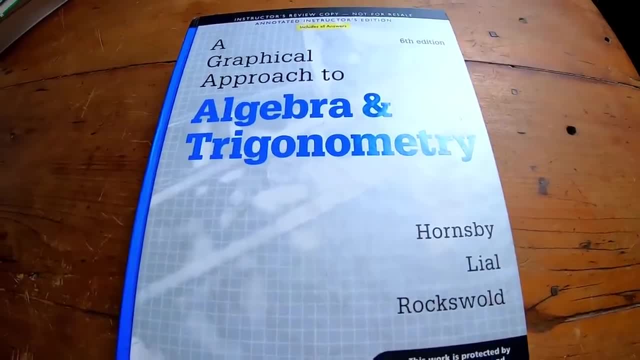 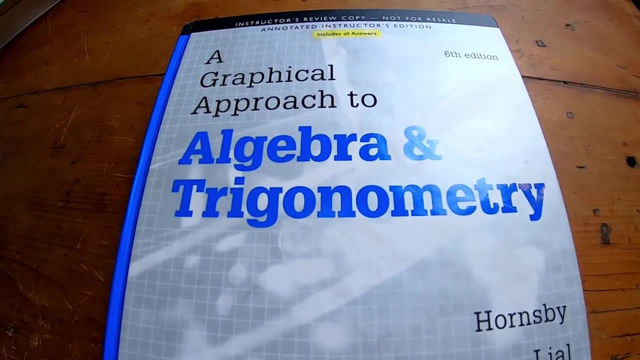 from college algebra, you can jump into this. This book is typically used to teach a course called pre-calculus and also trigonometry. in the US, Pre-calculus is like algebra. It's like college algebra but it's harder. So you do like more things. You do more things with inequalities. 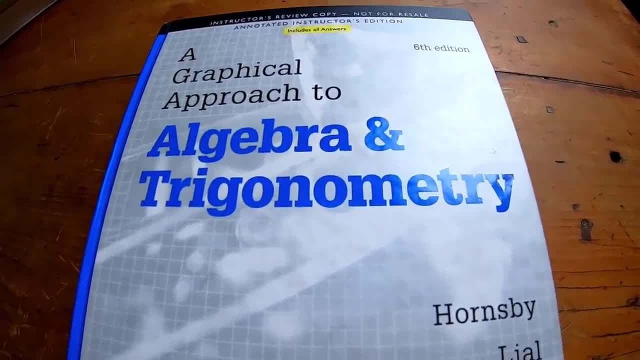 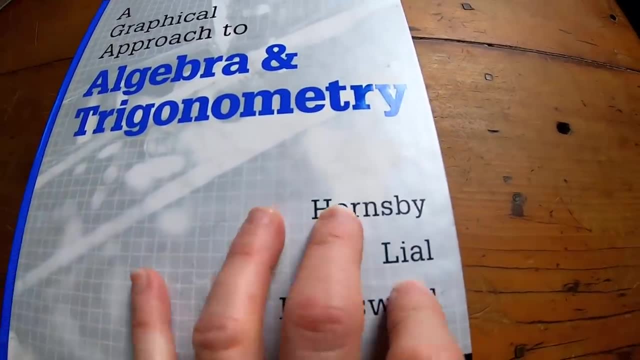 You do some stuff with numbers. You do some stuff with numbers, You do some stuff with matrices. It's just a little bit more challenging than algebra. So in theory, you could start with a book like this. This is the one by Hornsby, Lyle and Roxwold, And this is good because it's 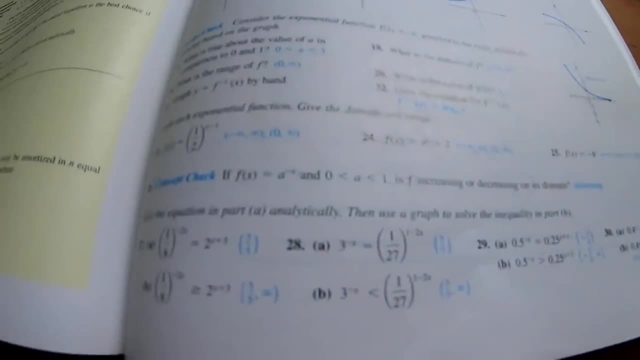 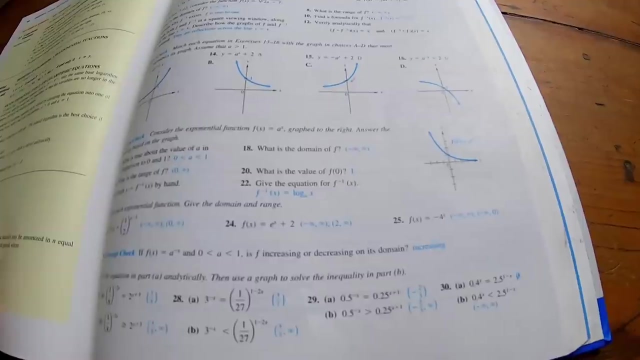 the instructor's edition, So it actually has answers to every single problem right next to the exercise, which is really convenient. And this book has everything right: It's got conic sections, It's got matrices, It's got algebra stuff. It's an awesome book. So, again, this is 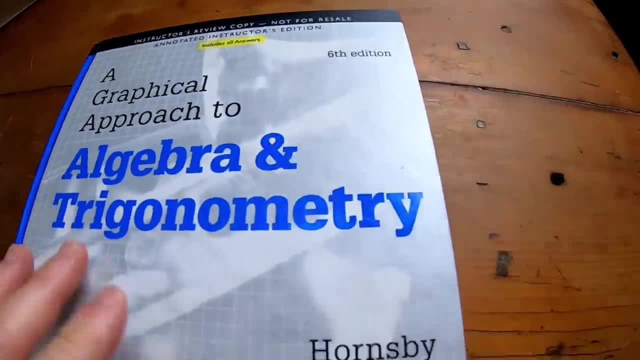 the book Graphical Approach to Algebra and Trigonometry, And it's the one by Kaufman, It's the one by Hornsby, Lyle and Roxwold, And again, you could in theory skip all the. 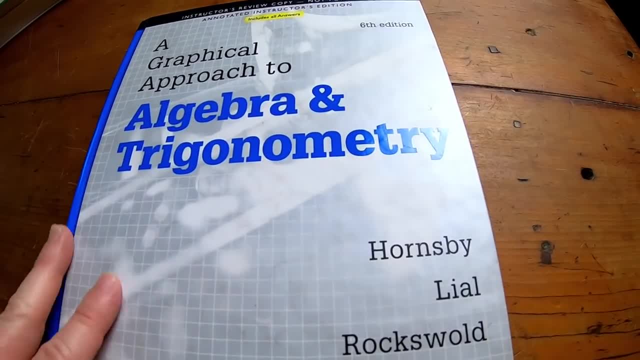 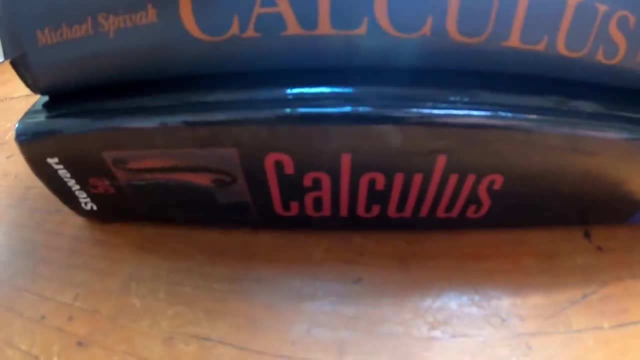 pre-algebra books. skip all the college algebra books and start here. So if you know some basic algebra, this is a good place to start. And we have finally arrived at calculus. So the book on the bottom you see here is Calculus by James Stewart. This is a common book. It's probably the 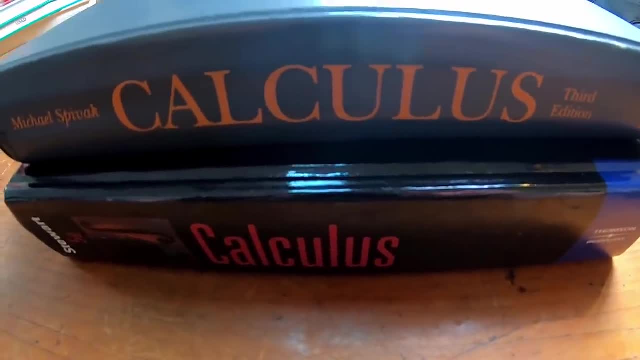 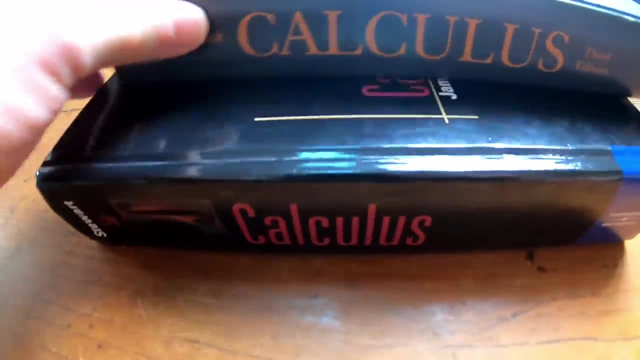 most popular book in the United States that's used to teach calculus And in Canada. James Stewart was a Canadian mathematician. He passed away several years ago, So this is a good book- This one Calculus for people who are going into engineering or if you just want to learn. 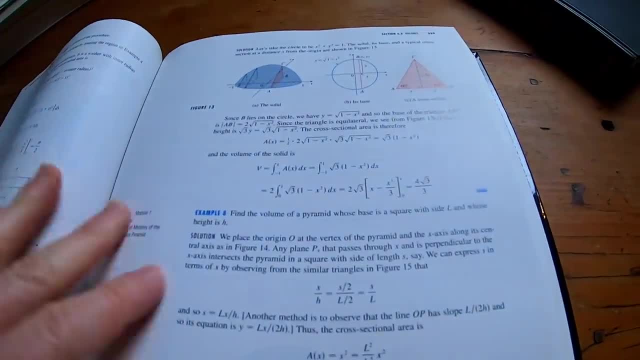 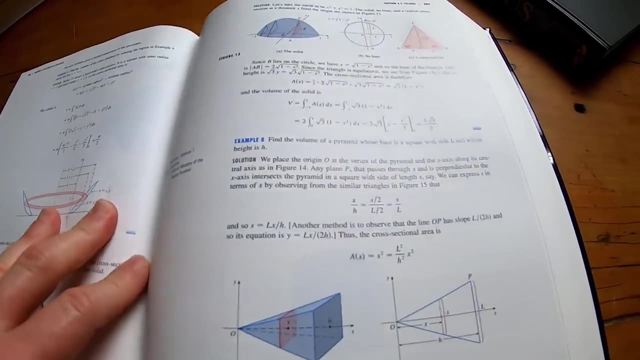 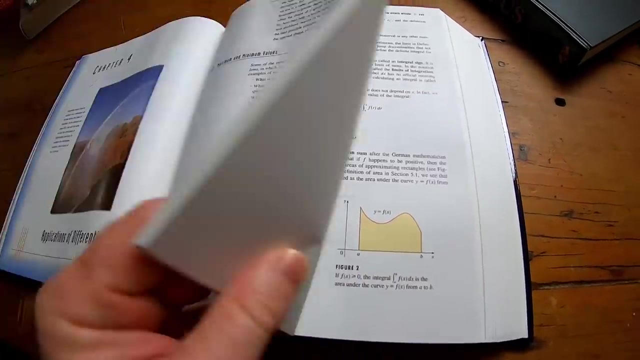 just basic calculus. It's got tons of problems and tons of pretty good explanations. A lot of people don't really like this book, but it's hard to find a book comparable to this one. Another good one is the book by Larson, So again worth owning a copy of this book. You can get a used. 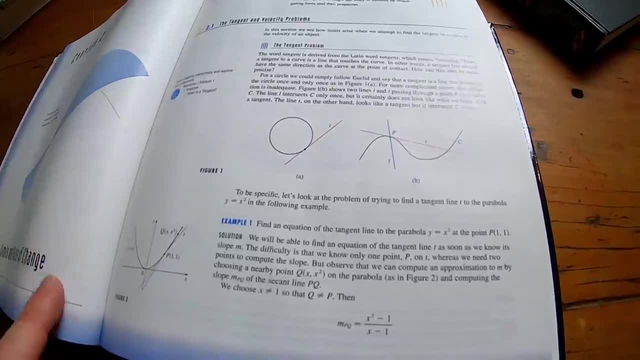 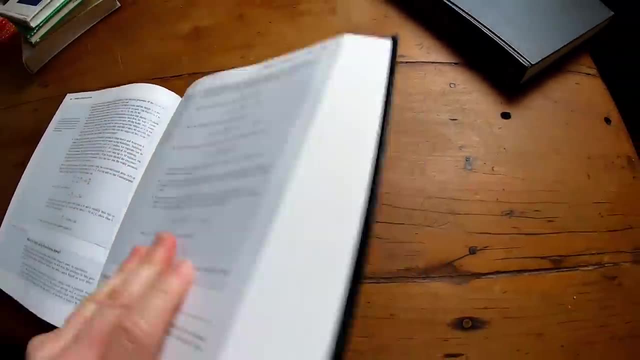 copy And typically, in the US at least, the courses that are taught with this book are calculus 1,, 2, and 3.. So you could use this book to teach yourself those things. So what about this other book? This is a famous book. This is called Calculus, by Michael Spivak, And this has less. 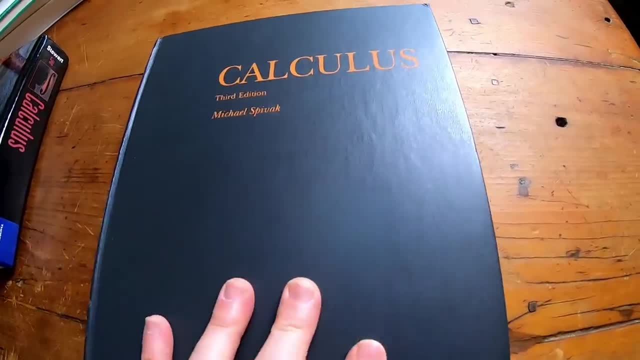 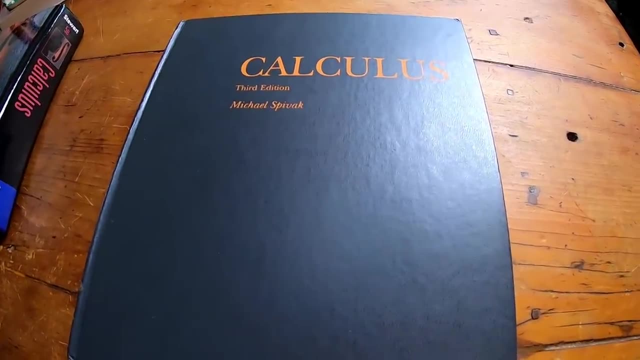 material than the Stewart book, but it's more advanced. And the beautiful thing is, if you've followed this video so far up to this point, you already know some logic and you already know some proof writing, And that is the number one thing that gets people hung up with this book. They'll 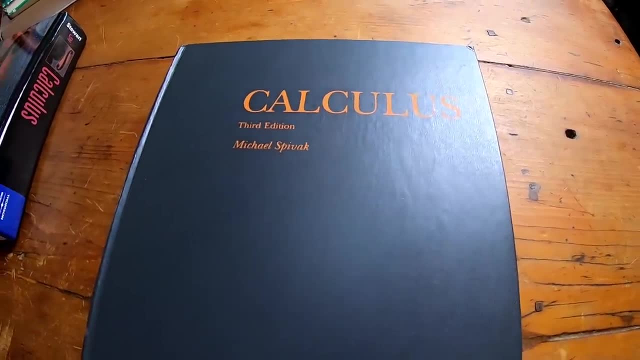 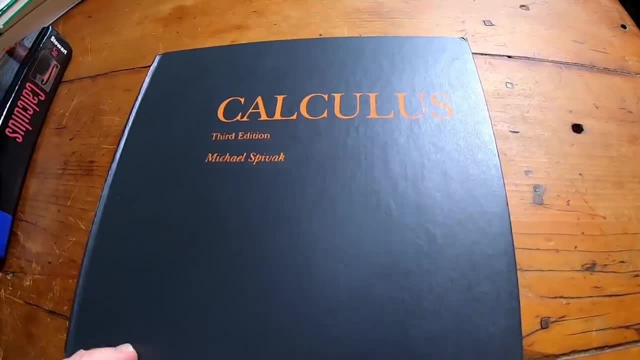 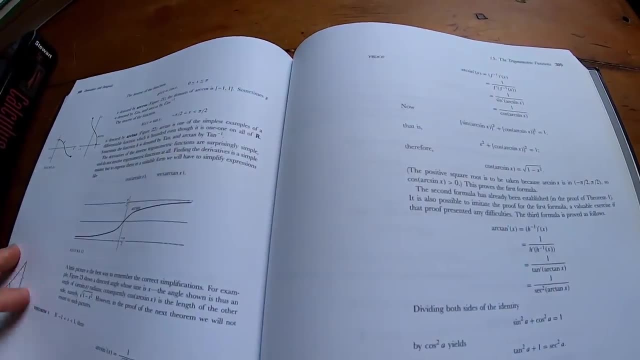 don't understand what's going on. What is Michael Spivak talking about? It's because those people lack the proof writing skills which we covered at the beginning of the video. So if you jump into this and you follow this order, you'll actually be able to read a book like Michael Spivak's. 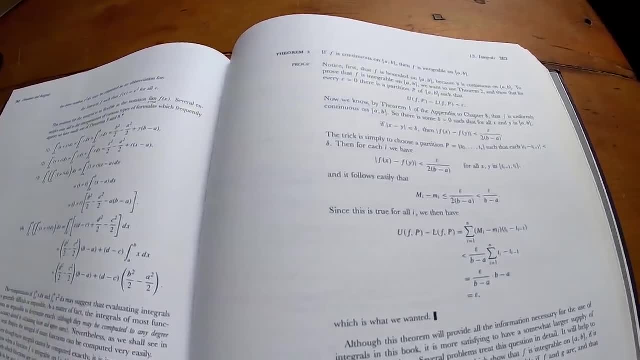 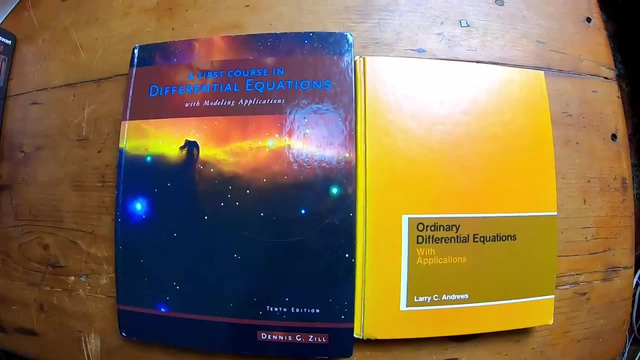 Calculus And you'll understand the trig that's in here. because you've learned some trig, So awesome book worth owning, especially if you know some sets and some proofs. Once you get through calculus, it's time to learn some differential equations, which are 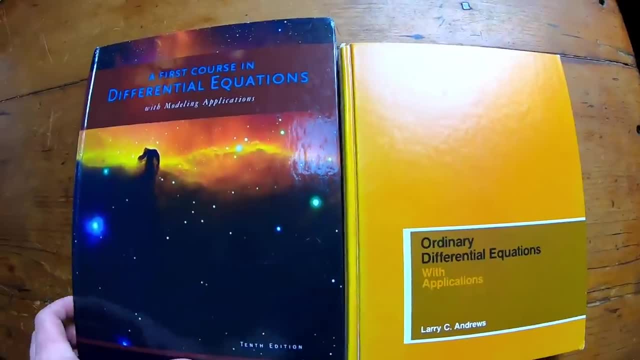 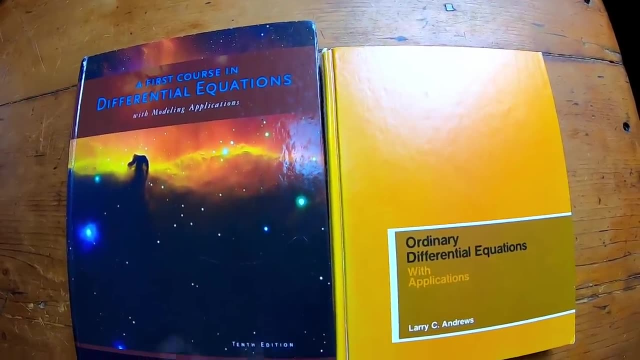 super awesome. The main thing for learning differential equations is that you know some integration. So if you go through a book like the Stuart book and you pick up all the integration techniques, that will help you a lot in a course like this. So this is the book that I use to teach. 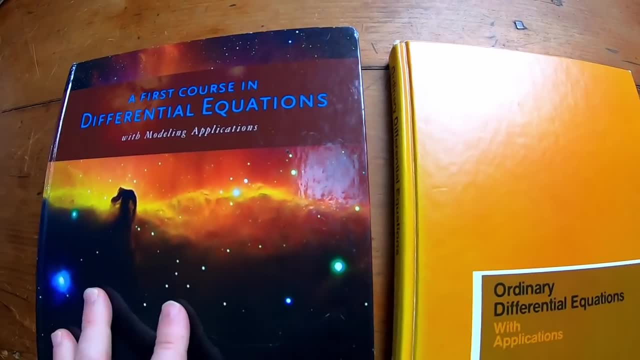 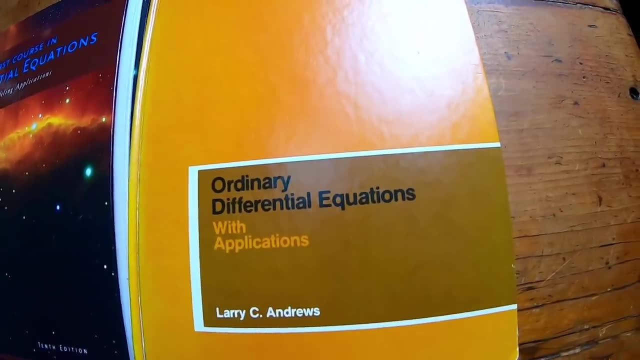 differential equations, So I'm biased. This is the one by Zill. It's an okay read. This one is a bit easier. This is the one by Larry Andrews- Not a very popular book but it's pretty good for beginners. It's called Ordinary Differential Equations by Larry Andrews. 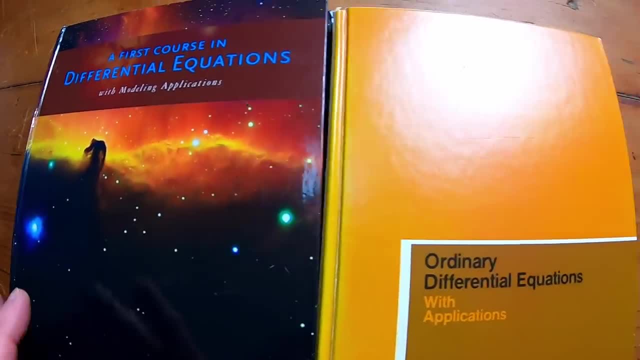 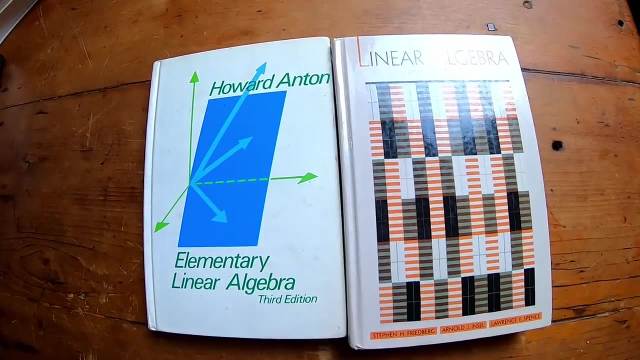 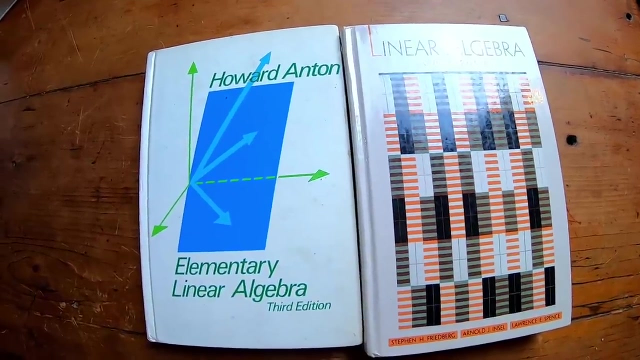 So, again, differential equations is a good next place to be. There's many more books. I'm trying to keep this video short, so here's two good ones. Okay, so now you know how to write really basic proofs. you know some basic logic and you know a little bit of calculus. And again, you don't have to be a master to jump into this stuff. 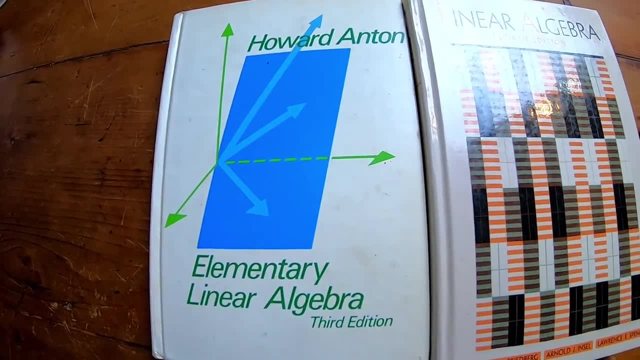 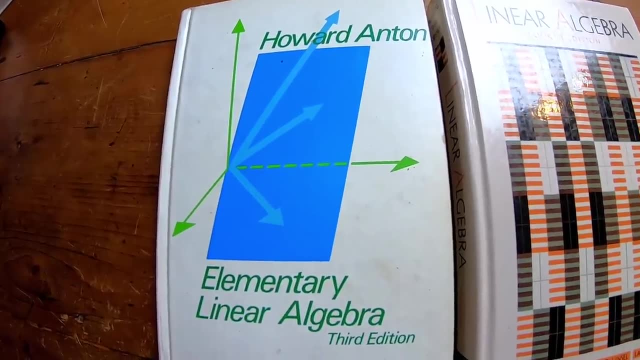 So now it's time for Linear Algebra. So this is the book by Howard Anton: Elementary Linear Algebra. I like this book for beginners because it's very consistent with what you would learn in the first place. This is the book by Zill: Elementary Linear Algebra. I like this book for beginners because it's very consistent with what you would learn in the first place. 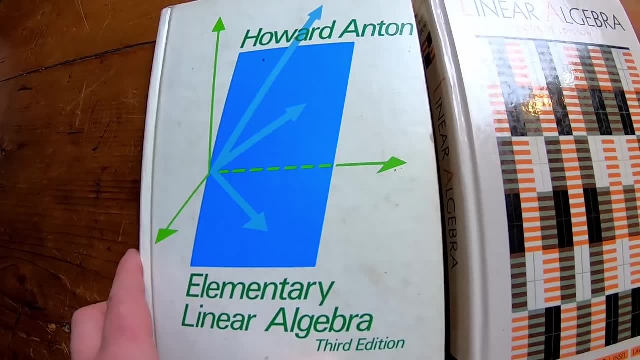 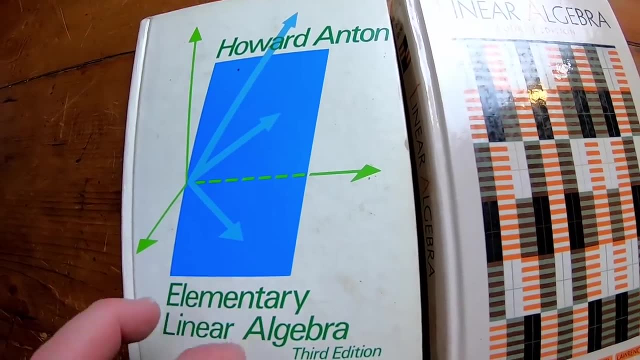 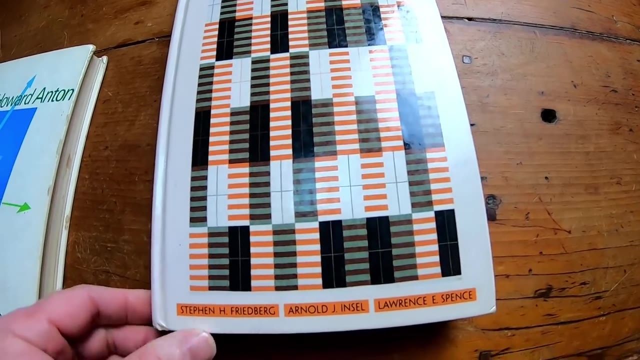 The exercises are very similar to like the test questions you would see in a college-level course. It's really really good for beginners. It goes along very well with what's taught, So that'll help you get an A in your class. This one is a much harder book. It's a dryer book, It's a much more rigorous book, but it is still worth owning. It is the one by Friedberg, Insell and Spence. 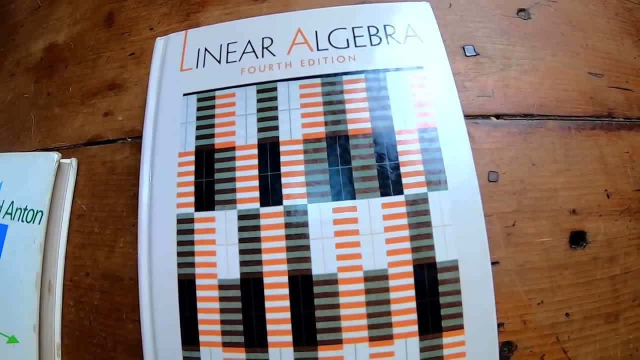 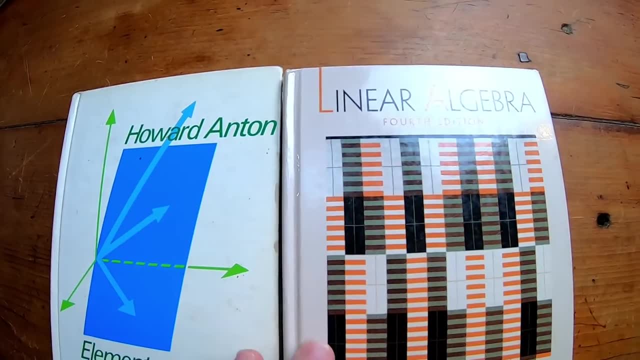 And this one is proof-based, but remember you have proof-writing experience, even just a little bit, because that's where you started. So both books are worth owning. And again, you would just try to learn as much linear algebra as you can in this next step. 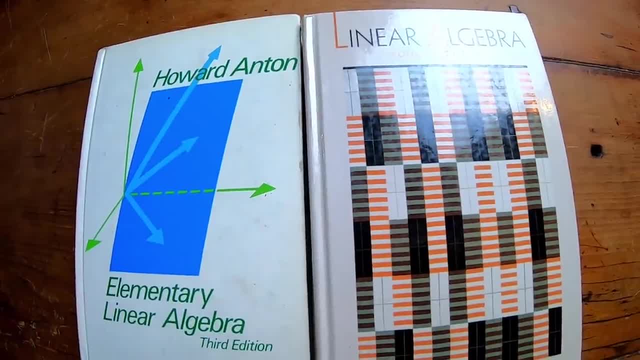 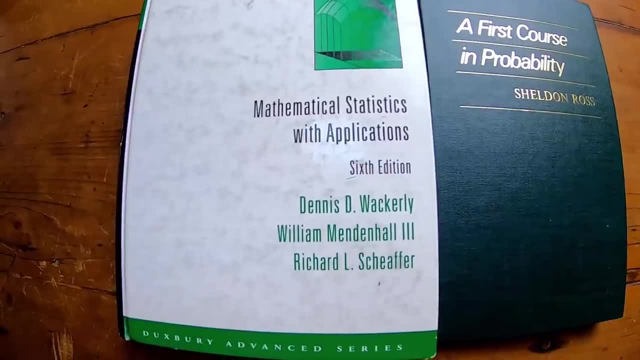 You don't have to master it before going to the next step. Let's keep going. At this point it's like the world is open because you know how to write basic proofs, you've made it through some calculus and you know some basic linear algebra. 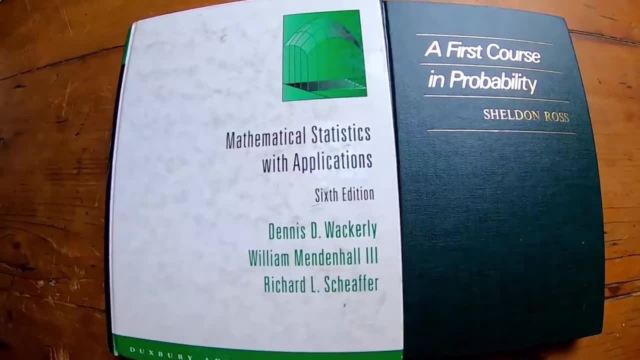 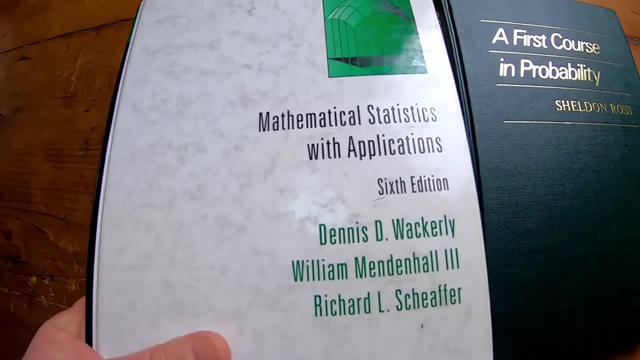 So now, in theory, you can learn almost any math subject that's taught at the undergrad level. So this is a book on mathematical statistics. So if you're interested in statistics, this is a really solid choice And this is an investment. 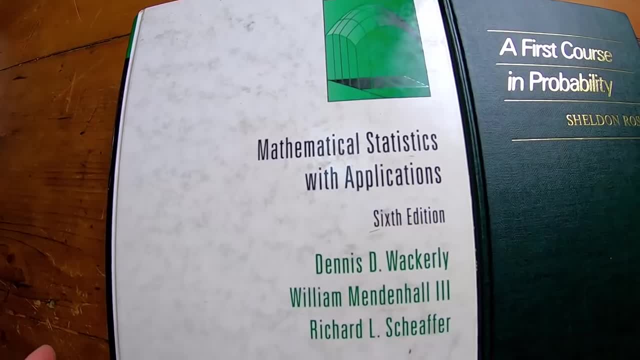 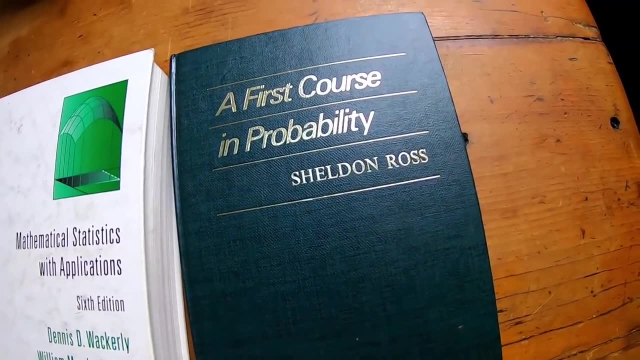 It's an advanced book but you know what. It's okay, You're at an advanced stage, You know calculus and this book requires calculus for some portions. This one also requires a little bit of calculus for some portions and it's called a first course in probability. 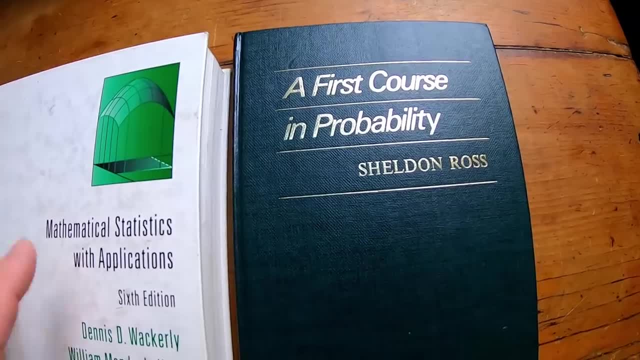 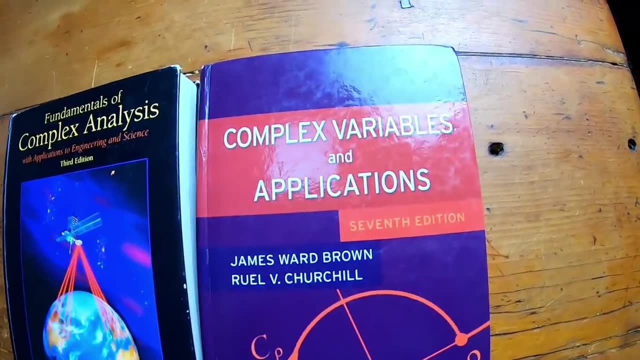 But again, a lot of this stuff can be done without calculus, but the fact that you know it will let you get through giant portions of these books. A very fun transition might be to jump into complex variables or complex analysis. That's basically calculus with complex numbers. 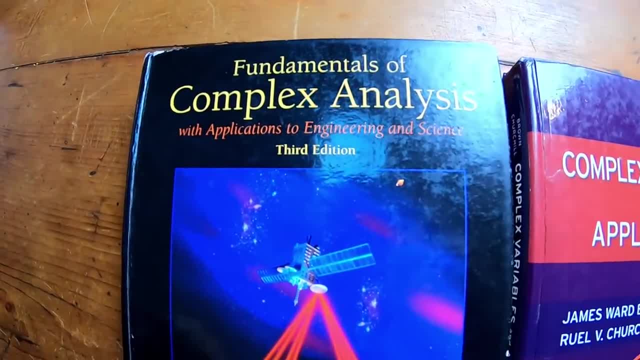 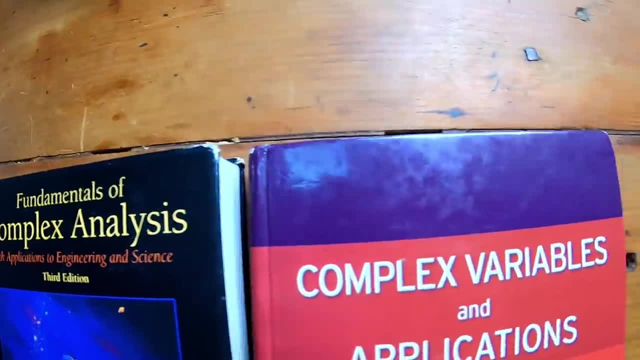 So in theory, you could actually skip differential equations and jump into this, Although I think it's better to learn differential equations first. It's fun, It's worth it. But this again, if you want to jump into this, once you know some calculus you can just jump into this. 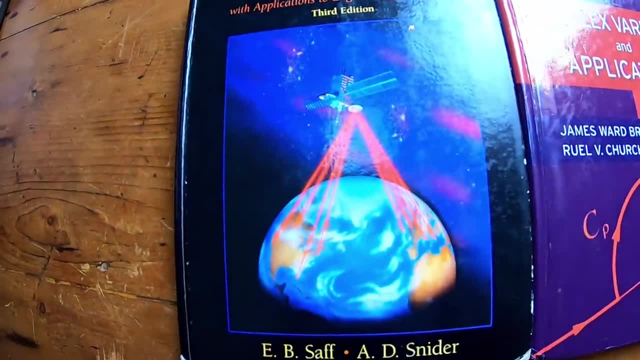 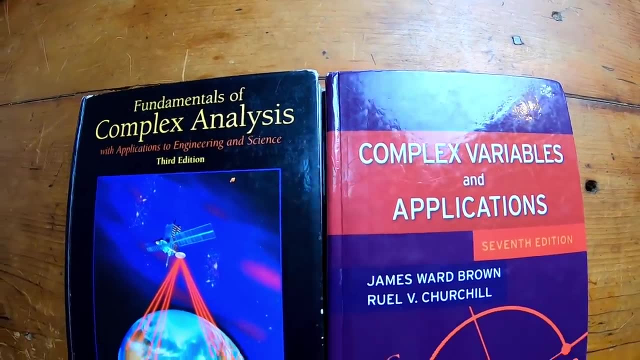 And you already know some, if you're at this point. So this is the book by Saff and Snyder and this is the book by Brown and Churchill. Both are pretty much the same. They're both excellent beginner books in the study of complex variables. 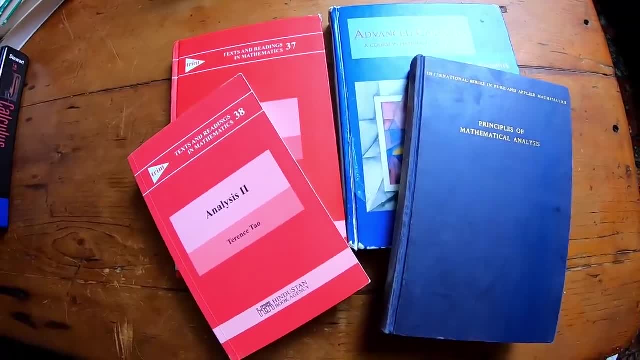 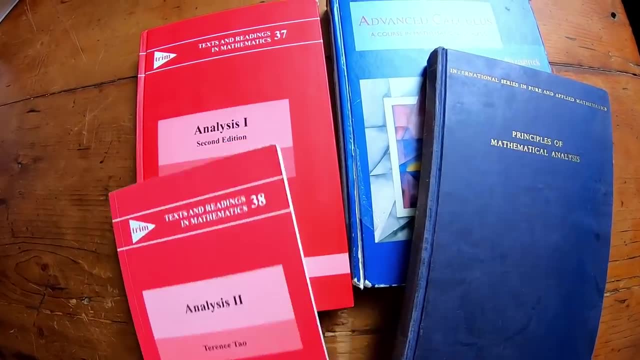 Real analysis is often thought to be complex. Real analysis is often considered the bane of math majors. This is probably one of the hardest, if not the hardest, class math majors take. You can actually learn that now if you're self-studying. 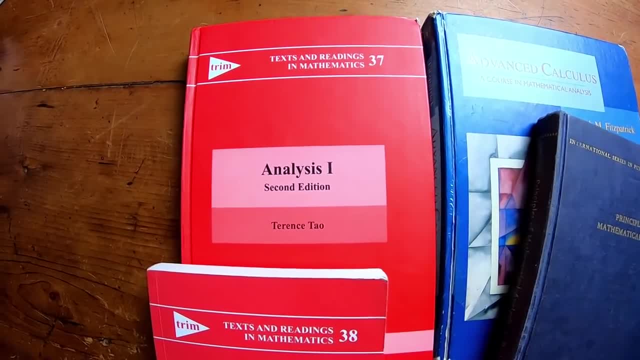 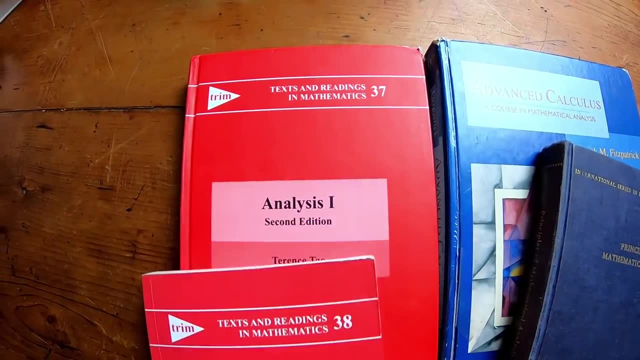 So again, you can just jump into this. after linear algebra. This is the book by Terence Tao. This is analysis one and analysis two. Really good for reading, Really good examples in these books: Extremely enlightening, Much more readable and much more interesting than these other two books. 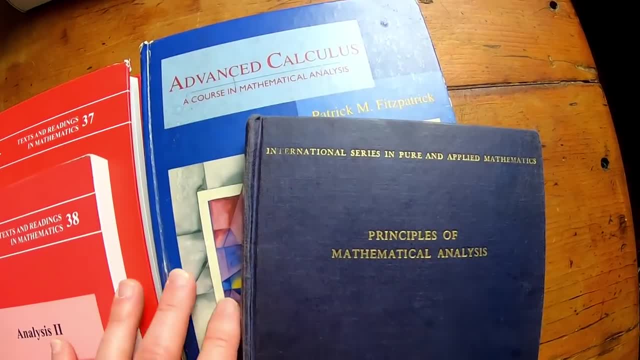 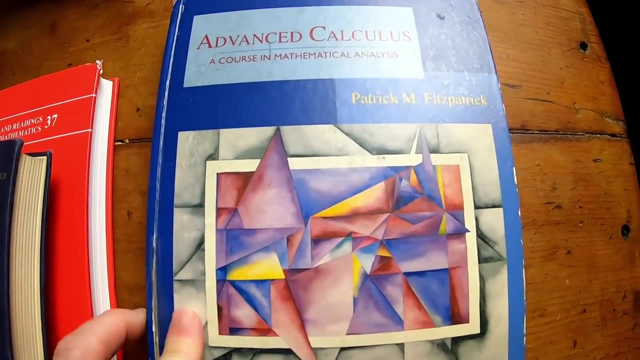 However, these other two books are a little more standard And they're still recommended. This is the one by Fitzpatrick: It's really good for beginners who are trying to learn advanced calculus. And this is the classic book by Rudin. It's called Baby Rudin. 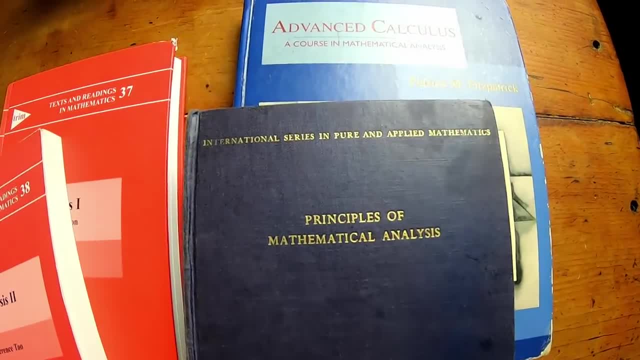 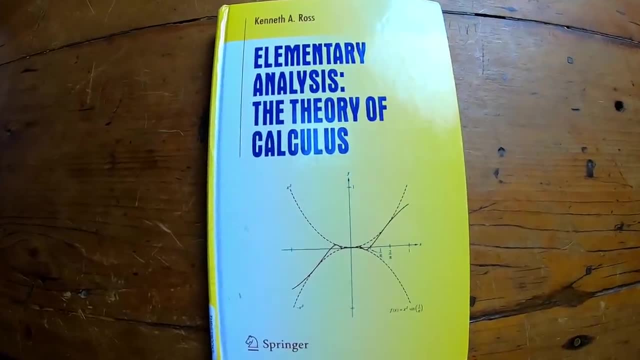 That's the nickname it has, And it's Principles of Mathematical Analysis. So any of these books would be good choices for beginning to learn some real analysis. One more- sorry, I forgot This is Elementary Analysis: The Theory of Calculus by Ross. 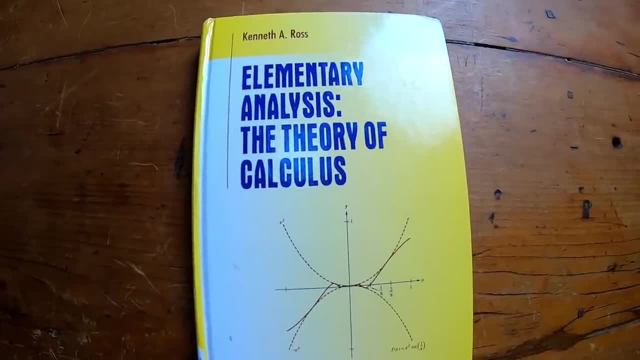 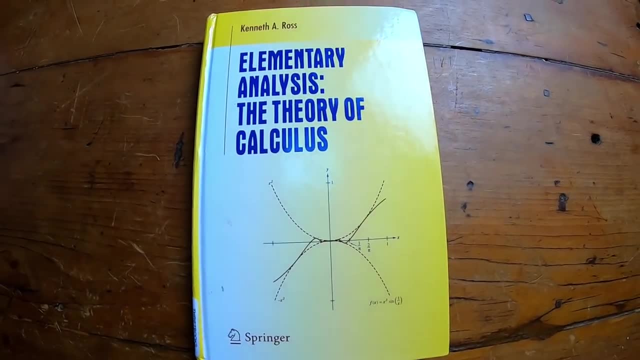 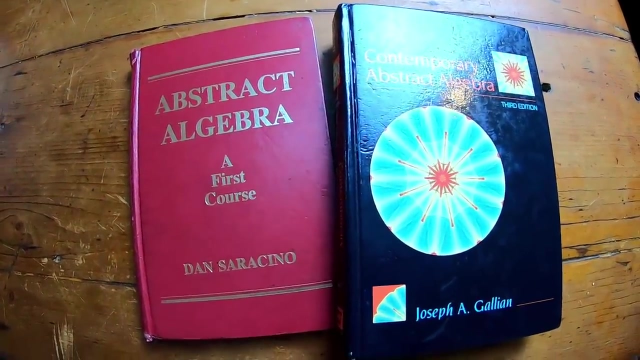 This one is very special Because he says: because he spends a great deal of time going into the proofs. So again, another solid choice for advanced calculus, aka real analysis. Another possibility that you could jump into now is Abstract Algebra. So Abstract Algebra is like the study of groups, rings and fields. 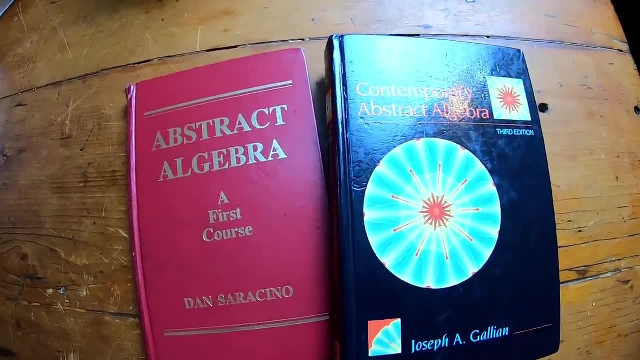 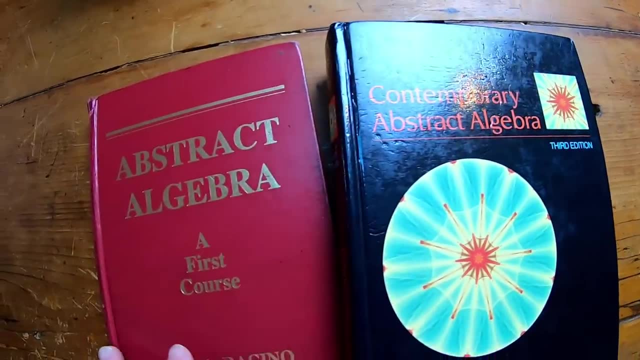 So you look at like a set with some like basic properties And it's really proof-based. So Linear Algebra is a good course to take before these, Because these are very, very proof-based courses. This is my favorite beginner book on the subject. 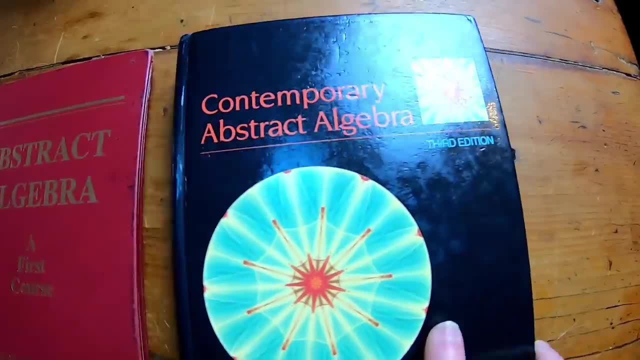 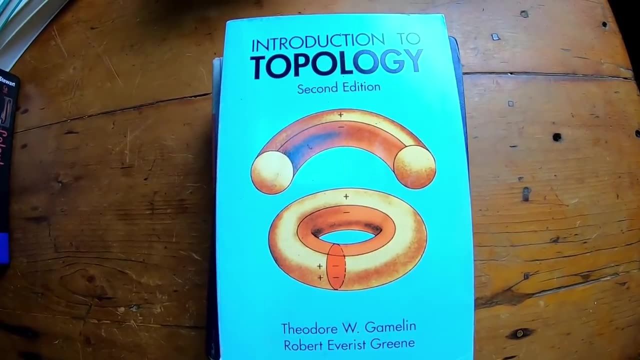 It's the one by Sarah Chino And this is the book by Galleon, Another good beginner book for Abstract Algebra. Okay, let's look at a couple more subjects that you can actually learn now. So Topology: I just picked a book I have on Topology. 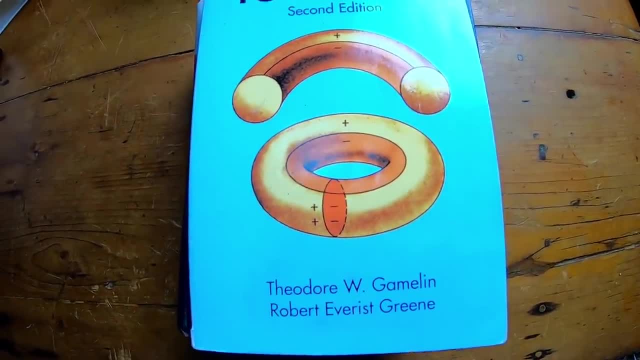 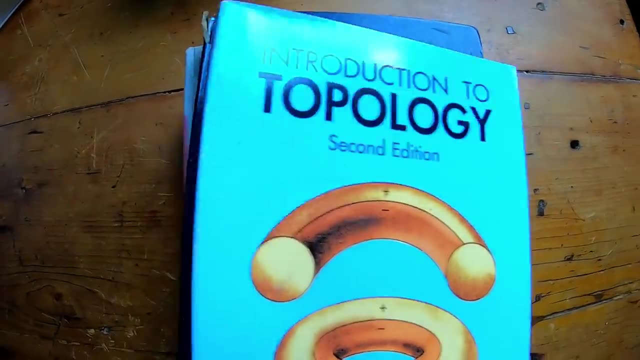 This one has full solutions to all of the problems. This is the one by Gamelan and Green. It's a great book And it's a Dover book, So that means it's cheap. It's only a few dollars on Amazon. Let's see what's below it. 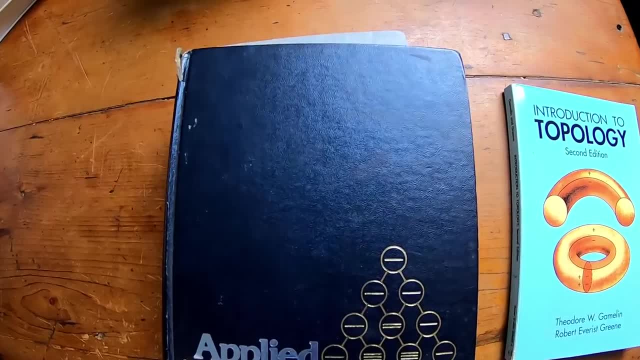 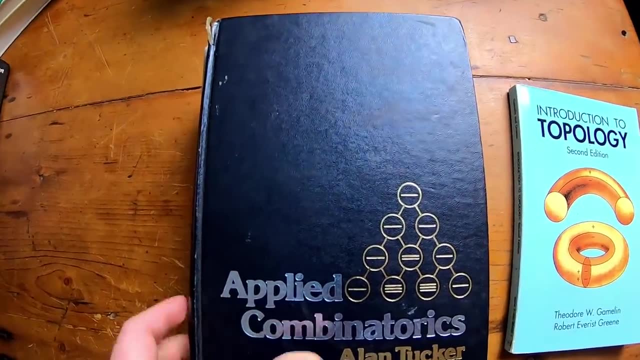 This is a book on combinatorics. This is the one by Alan Tucker. This is an okay book. The good news is you will know some combinatorics because you started with those discrete math books, So a lot of what's in this book will be review. 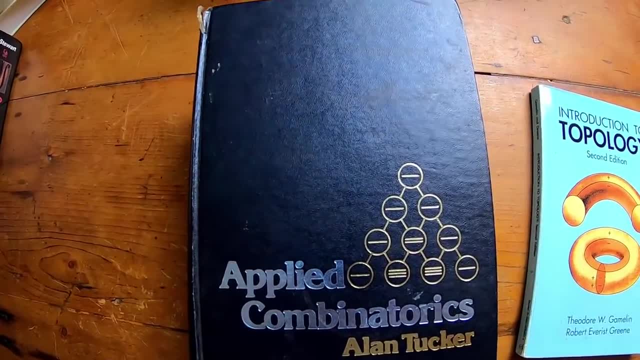 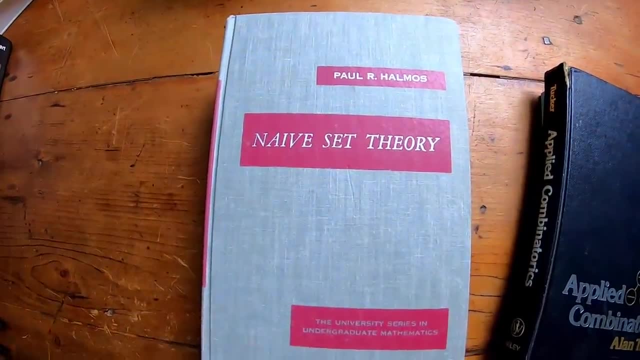 So, even though this is a little bit more advanced book, you have some background in it because you started with this stuff. That makes it awesome What's below it- Naive set theory. So this is something that could have been studied. you know even near Linear Algebra. 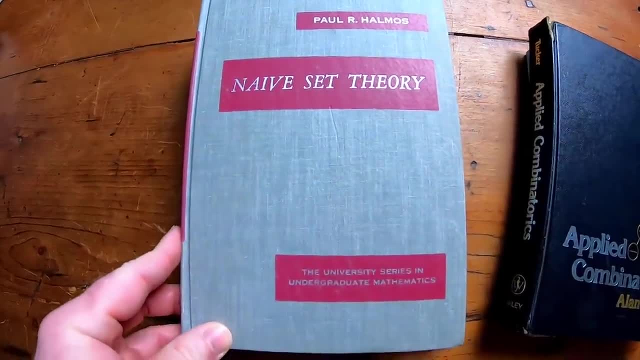 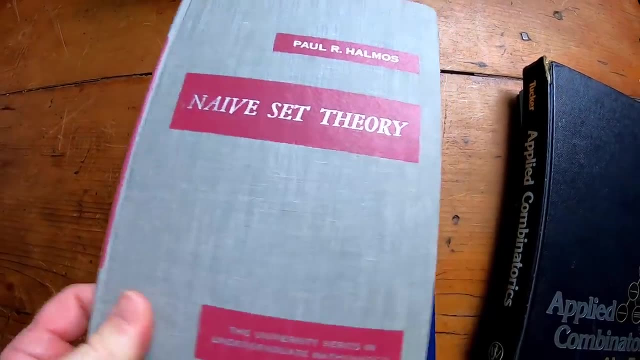 Set theory is not a very difficult subject. This is the classic book by Paul Halmos, who passed away several years ago. This is a very famous book. It's a little book. It's quite enjoyable. Again, it's naive set theory by Paul Halmos. 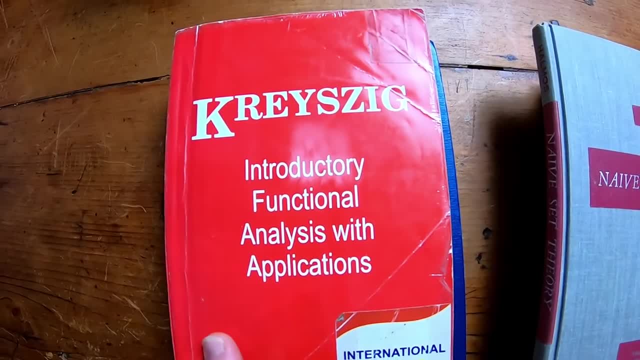 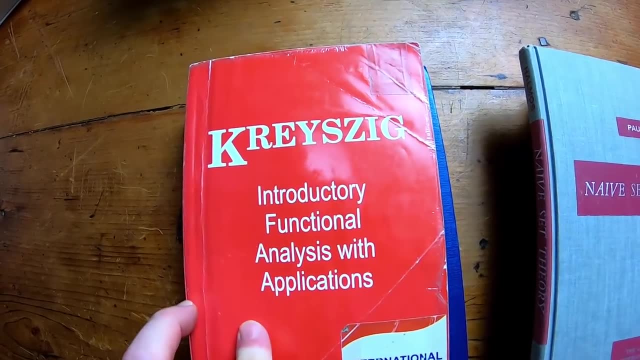 This is a book on functional analysis And, yes, in theory you could learn this stuff. You already know some advanced calculus, aka real analysis. You know how to write proofs. This is probably the easiest book on the subject. It's the Kreisig book on functional analysis. 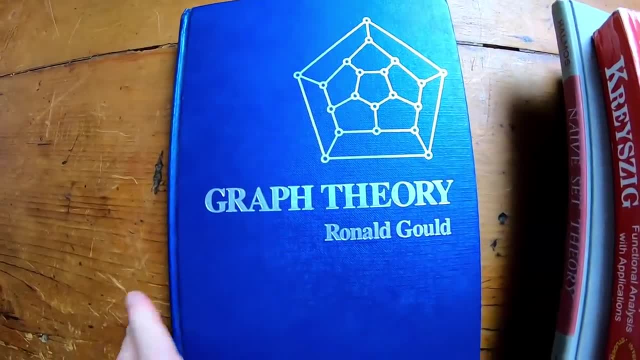 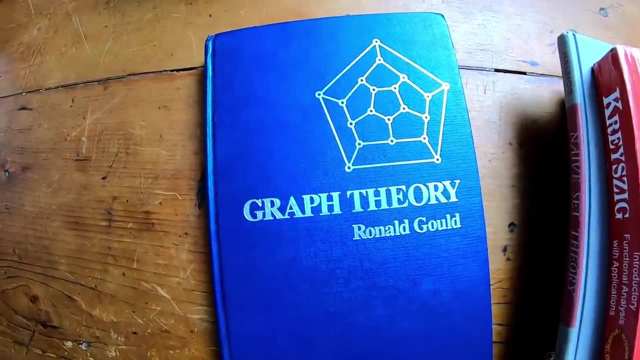 And what's below this? A book on graph theory. This is the book by Ronald Gould And again, you might already know some graph theory because you started with that discrete math. That's why I think it's such a good starting point. 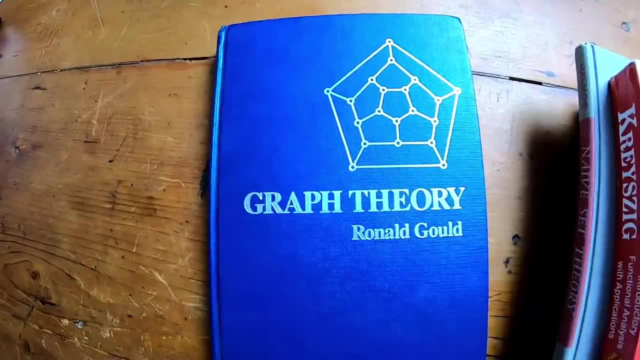 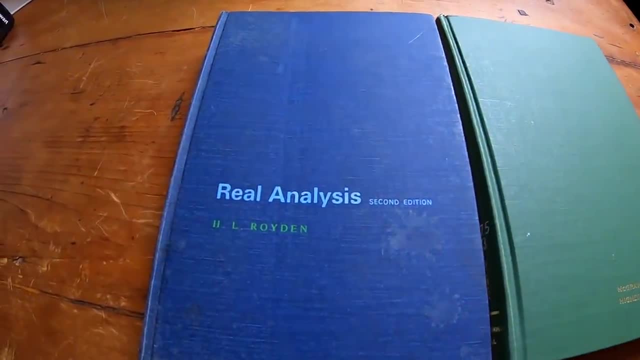 That's why I picked this order for this video. Let's look at some more stuff. If you really want to get into the higher level math, you could, You could do it. So here we have two famous books. This is the one called Real Analysis by Royden. 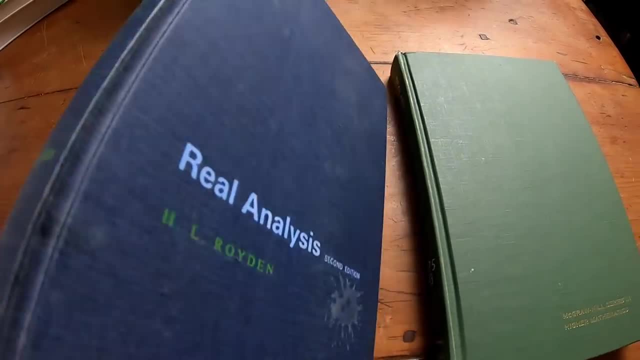 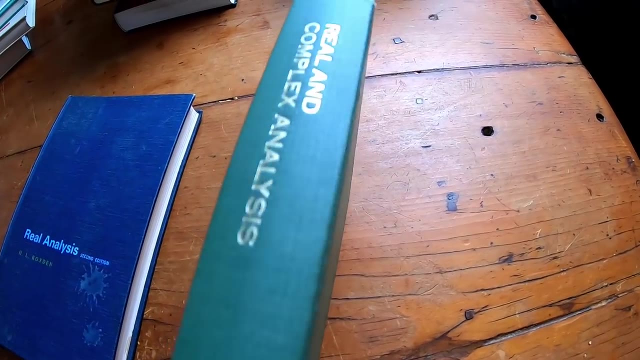 And this is a book on basically measure theory. This is gradual level mathematics, Really hard stuff, And this is the classic book nicknamed Papa Rudin. by Rudin It's called Real and Complex Analysis And this is the book by Rudin. 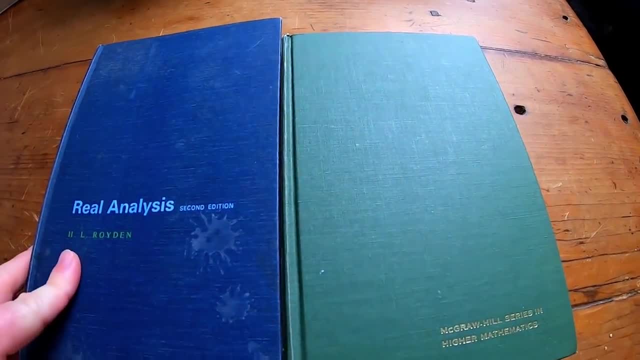 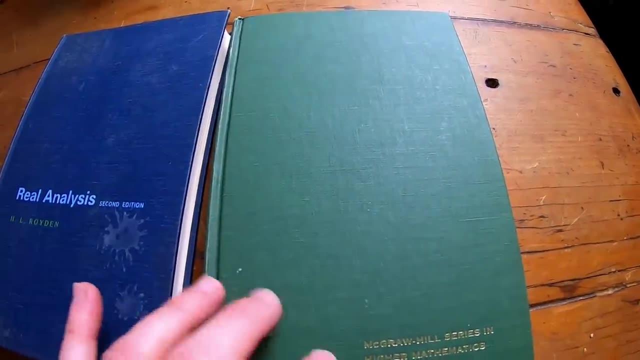 Both of these can be gotten quite inexpensively. perhaps I know the Royden book isn't so much money This one might have appreciated over the years. You know it's kind of a cult classic, But so is Royden, And I think Royden is a little bit better. 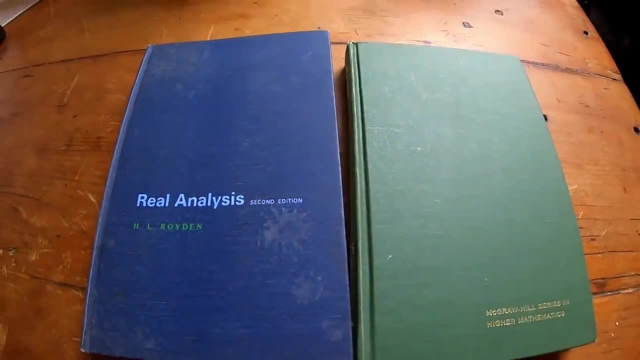 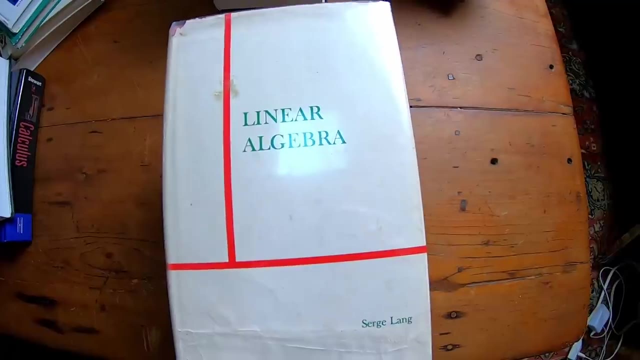 So both are good books For attempting to teach yourself some graduate level math. Let's take a look at some more books. So these are just books that I left out of the video that I had at the beginning in the video in the first scene. 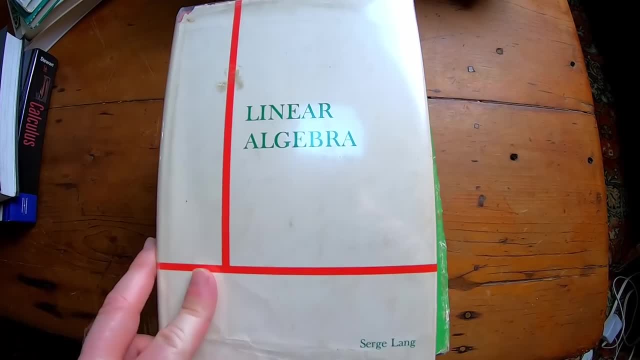 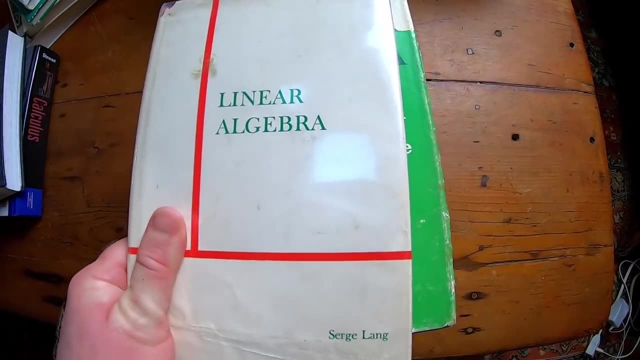 So let's just talk about them. So this is one on linear algebra. This is the one by Serge Lang, And this could have been another choice for learning linear algebra. I love this book. It's an excellent book And you can get it very inexpensively. 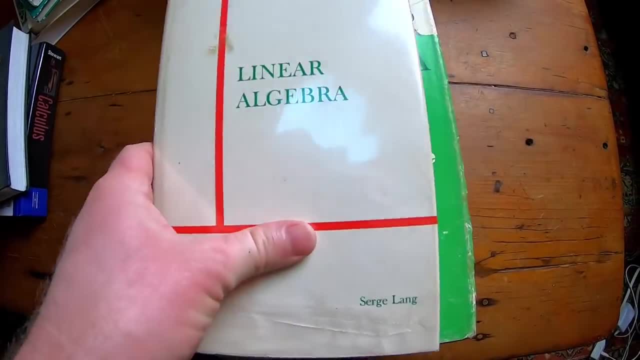 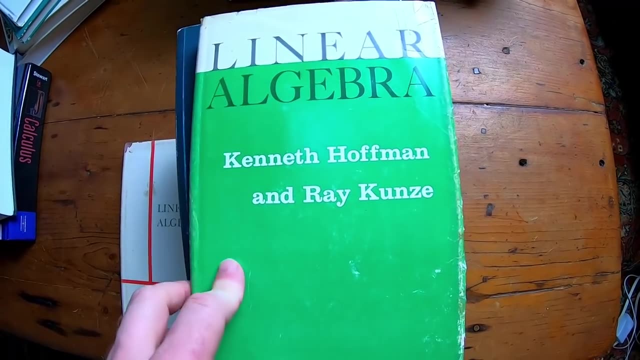 One of my favorite: Linear Algebra by Serge Lang. What's below it, Ah? Linear Algebra by Hoffman and Kunz. This is a classic. This is a book that was used at MIT, I believe, in the 60s. This is more like the Friedberg book. 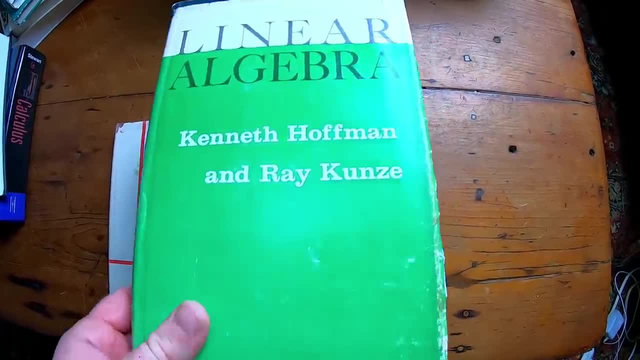 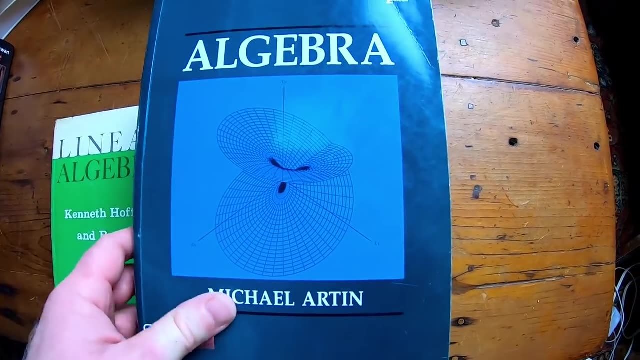 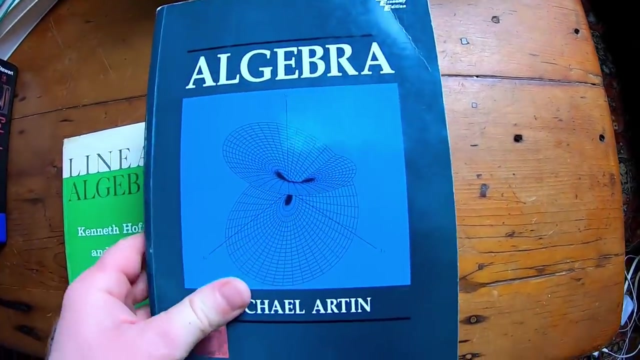 It's a proof based linear algebra book. This next one is Algebra by Michael Artin. So this is a great book on algebra. It takes a linear algebra centric approach to abstract algebra. So this is an abstract algebra book with an emphasis on linear algebra. 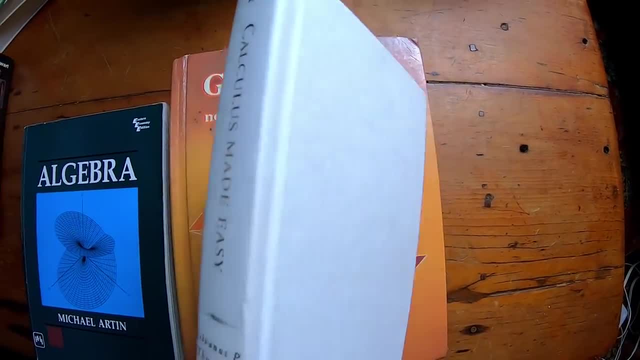 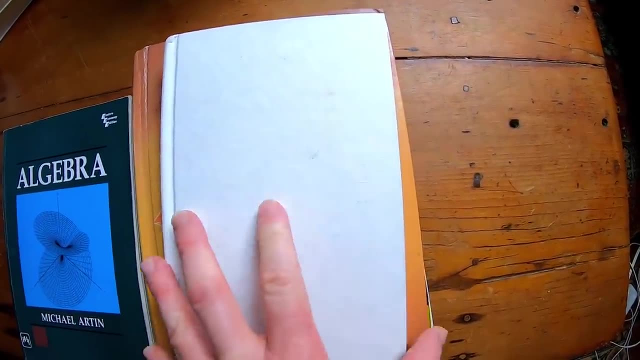 What is this book This is? This is Calculus Made Easy by Thomson. This is a book you read when you're laying in bed. I should have mentioned this one before, but this one's worth picking up. This is an old book, written, I think, over. 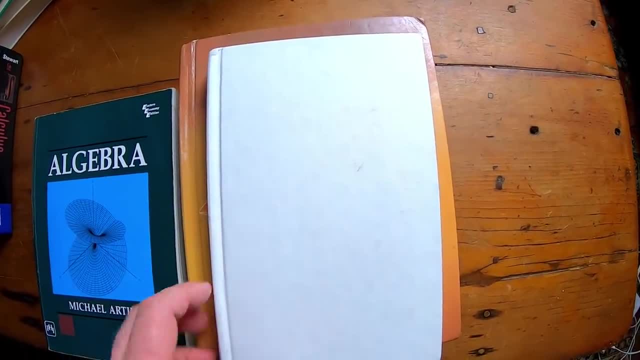 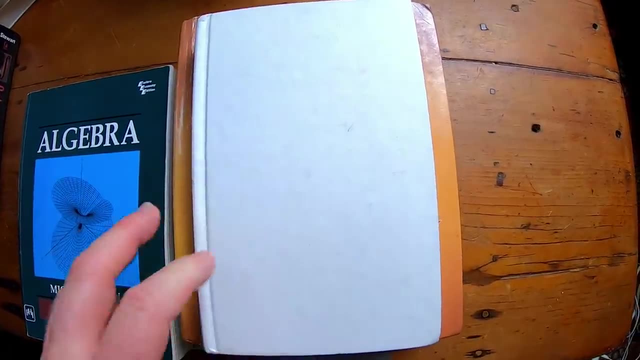 It's written a long time ago, I think, from the 1900s, early 1900s, And yeah, this is an awesome book for calculus and for understanding calculus. So you don't want to use this by itself to learn calculus. 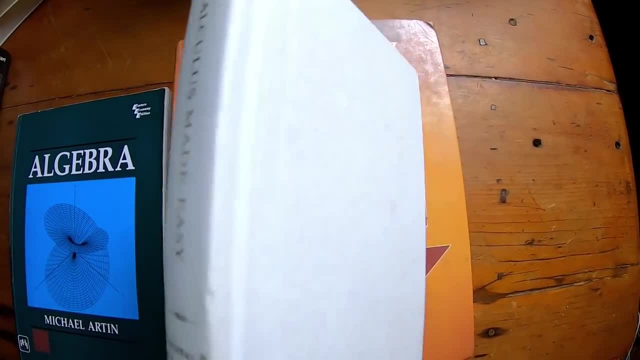 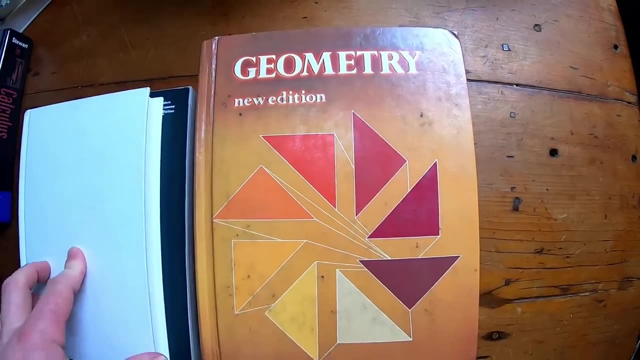 You kind of want to use the other book I recommended and then, like, lay in bed and read this one. This will give you some more intuition. Here we have a geometry book. That's right. I had nothing in this video about geometry, so I thought I should include a book. 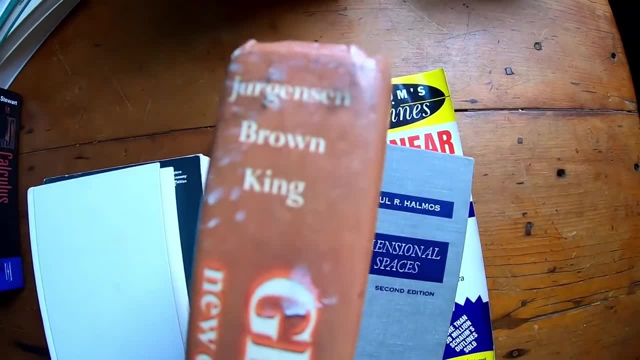 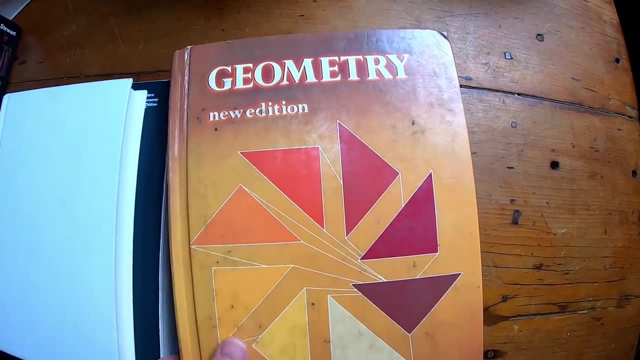 This is just a basic book on geometry and this is the one by Jurgensen, Brown and King. So just really, really basic geometry. You can learn this at any point, independently of any of the other topics. Here we have another book by Paul Halmos. 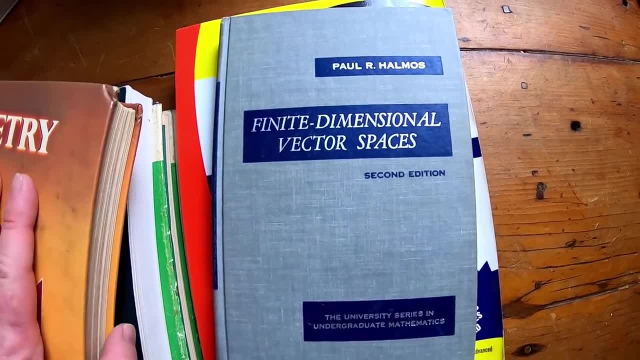 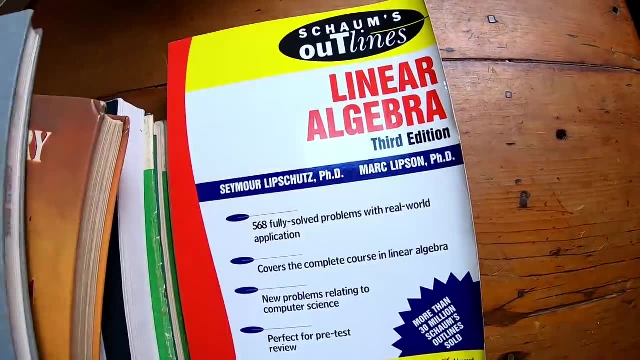 This is his linear algebra book. It's called Finite Dimensional Vector Spaces And this is something again that you can use to learn linear algebra when you decide to jump to that stage. And then another book on linear algebra. This is the Shams. 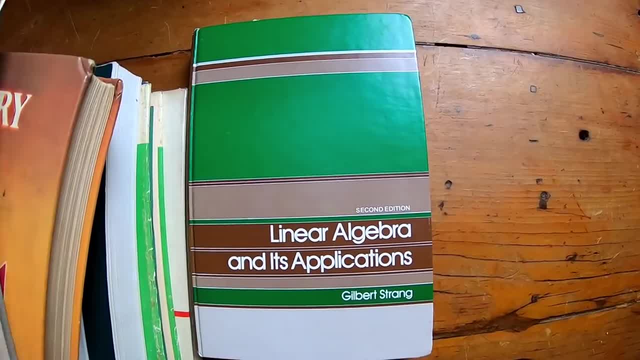 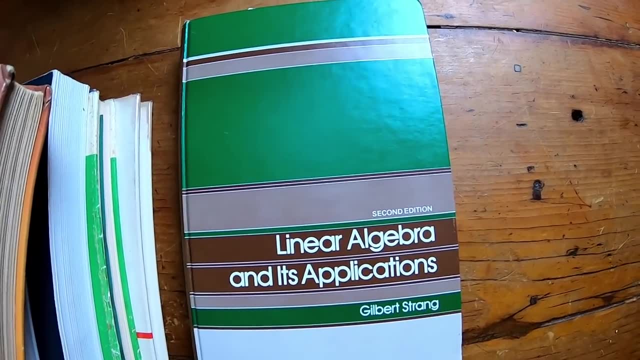 Again, just another resource to have. And then another book on linear algebra. This is the one by Gilbert Strang. That's the guy who has the MIT lectures and I think they're on YouTube also. Really cool, really cool guy. 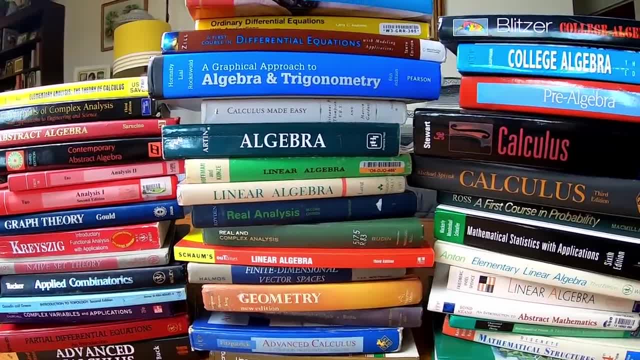 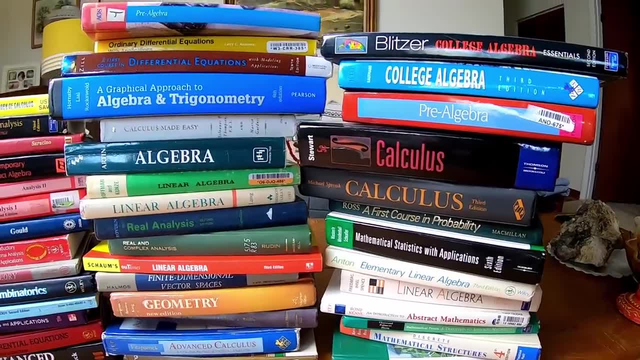 So those are the suggested ways of teaching yourself mathematics from start to finish, And again, you don't have to follow this particular order. And also keep in mind, when you're trying to teach yourself math, that math is hard and you're going to get stuck. 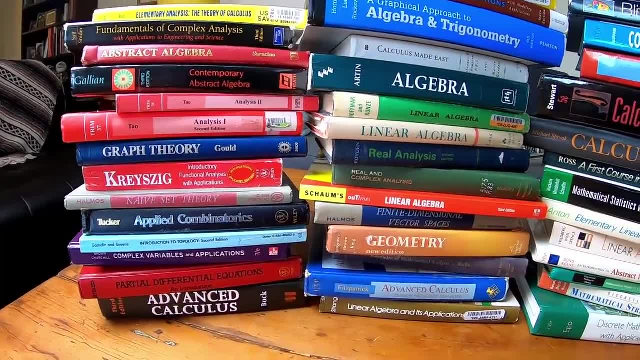 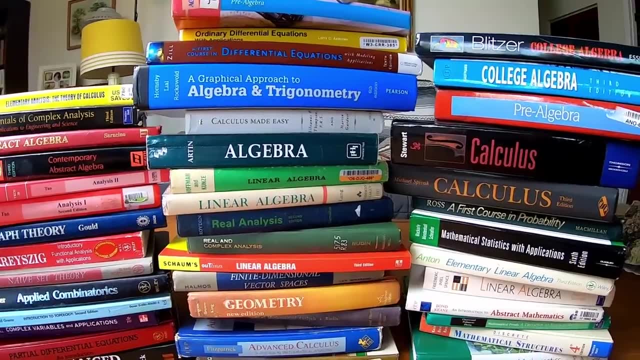 You might not understand everything, and that's normal, and that's okay and that's expected. So say you're learning calculus and there's just some stuff you don't get. It's okay. Feel free to move on and explore your interest, right? 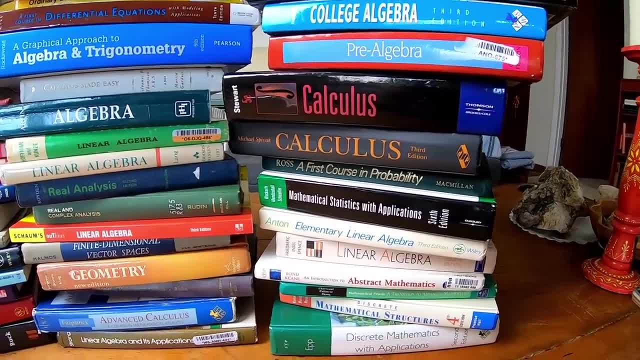 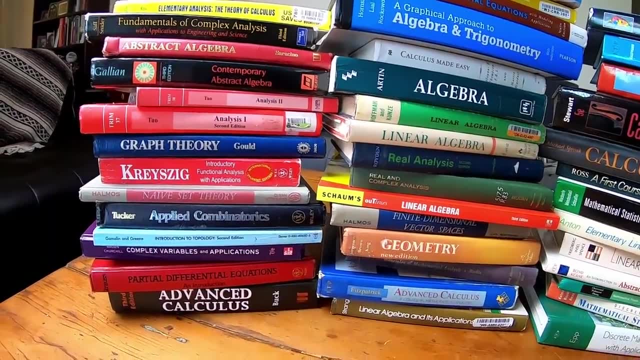 This video is about teaching yourself math. It's about learning for the sake of learning and, you know, enriching your life. It's about learning for mathematical knowledge, So I think it's the best way to do it. You know, you read what you enjoy.